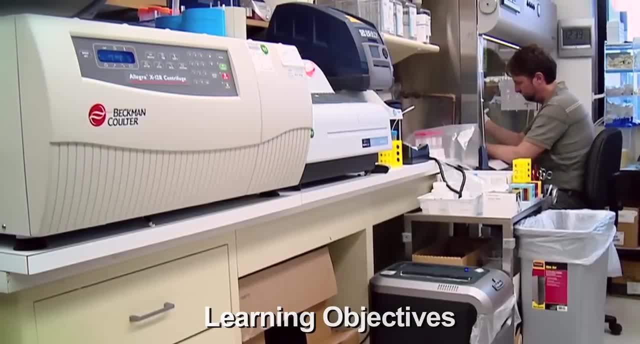 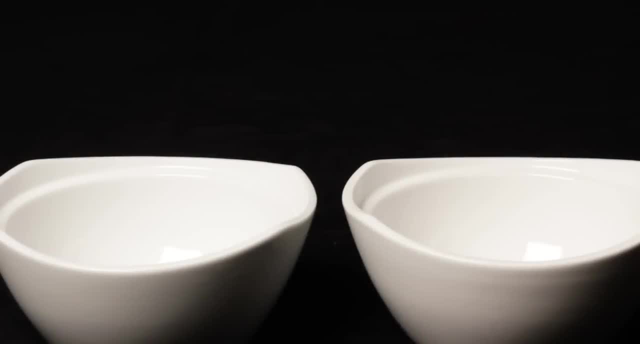 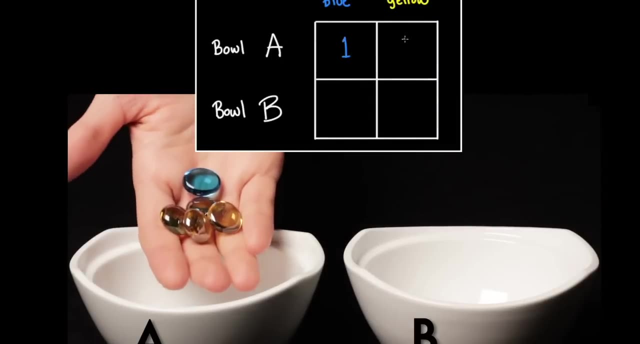 Then you'll be able to understand how conditional probability can be used to interpret medical diagnoses. How to Contemplate Conditional Probability? Suppose that in front of you are two bowls labeled A and B. Each bowl contains 5 marbles. Bowl A has 1 blue and 4 yellow marbles. Bowl B has 3 blue and 2 yellow marbles. 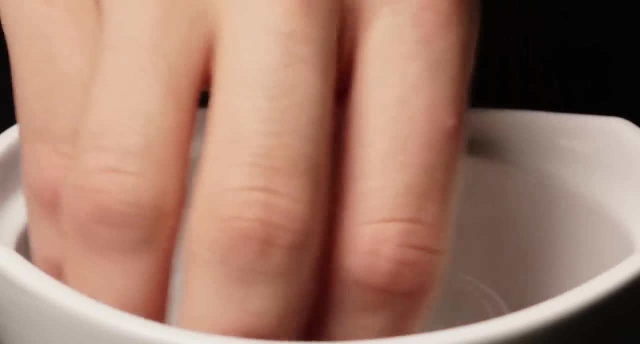 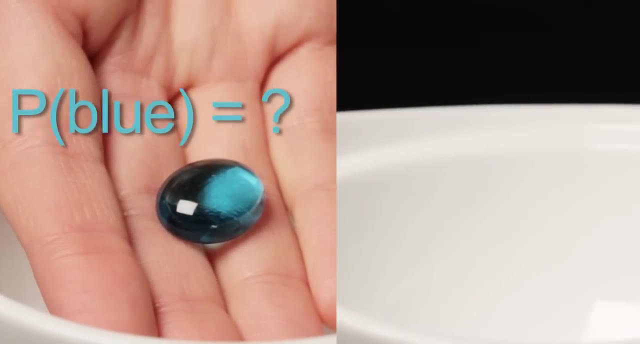 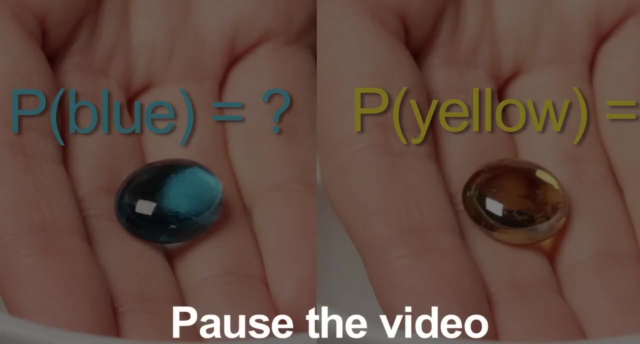 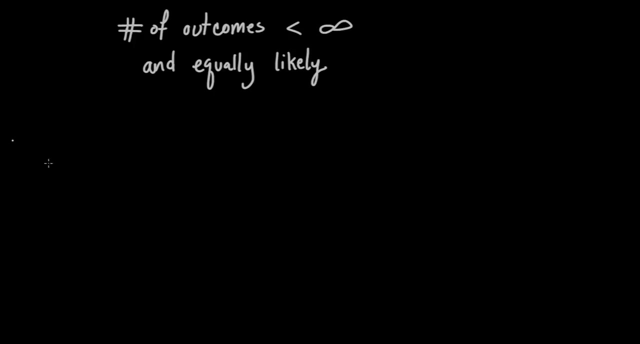 Now choose a bowl at random and draw a marble uniformly at random from it. Based on your existing knowledge of probability, of probability, how likely is it that you pick a blue marble? How about a yellow marble? Pause the video. When the number of possible outcomes is finite and all outcomes are equally likely, the probability- 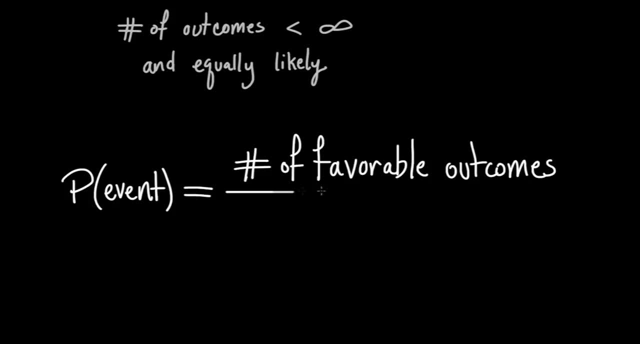 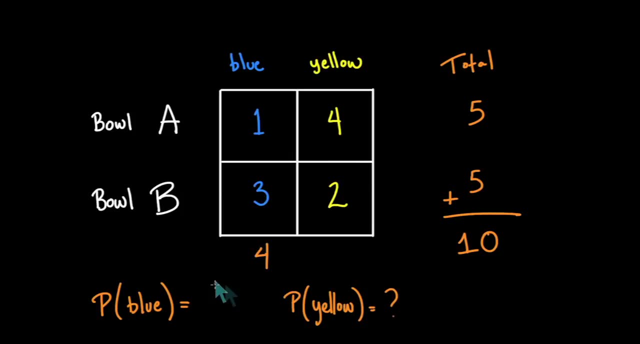 of an event happening is the number of favorable outcomes divided by the total number of possible outcomes. Out of the ten marbles you could choose from, four are blue, so the probability of choosing a blue marble is four out of ten. There are six yellow marbles out of ten total. 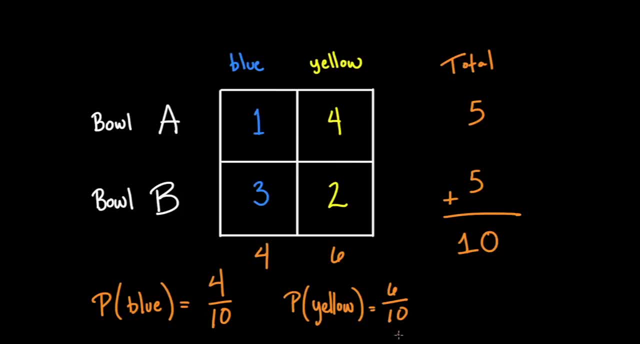 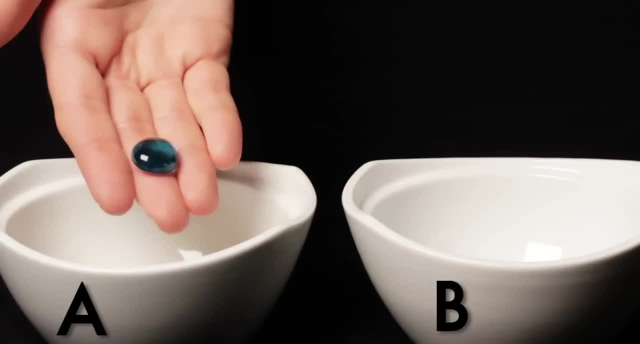 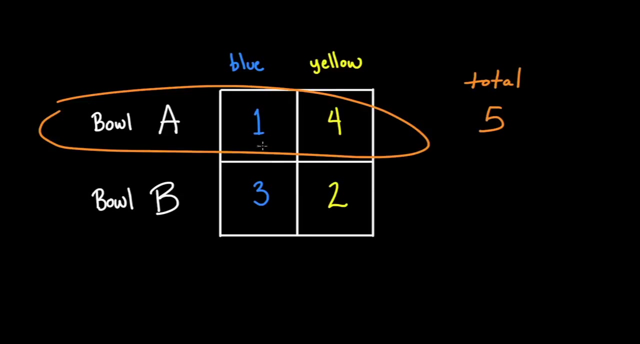 so the probability of choosing yellow is six out of ten. What if you must draw from bowl A? What's the probability of drawing a blue marble, given that you draw from bowl A? Pause the video. Let's go to the next slide. Let's go back to the table and consider only bowl A. Bowl A contains five marbles, of which 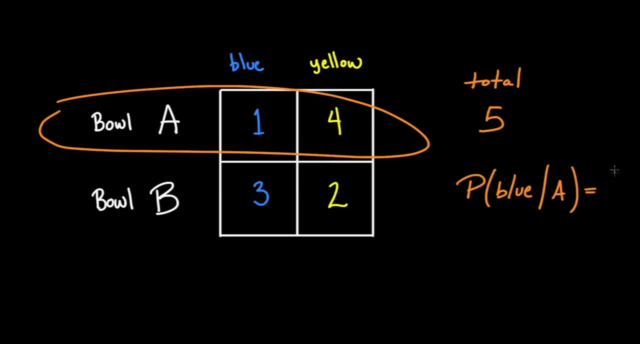 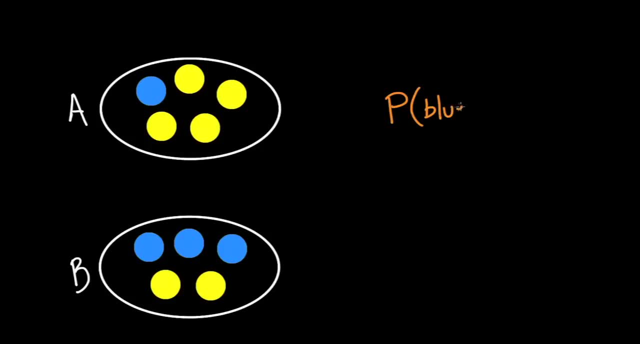 one is blue. so the probability of picking a blue one is one in five. Notice that the probability has changed. In the first scenario, the sample space consists of all ten marbles because we are free to draw from both bowls. In the second scenario, we are restricted to bowl A. Our new sample space consists of: 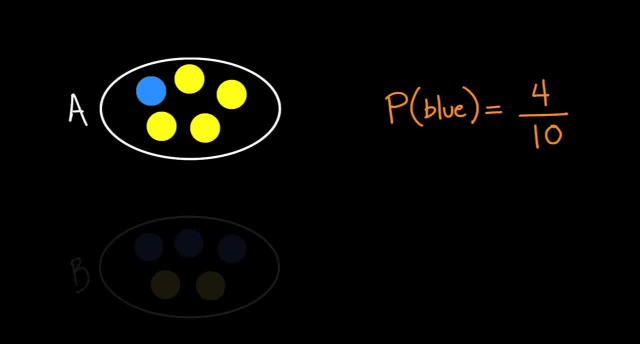 only the five marbles in bowl A. We ignore the marbles in bowl B. Restricting our attention to a specific set of outcomes changes the sample space and can also change the probability of an event. This new probability is what we call a conditional probability. This is 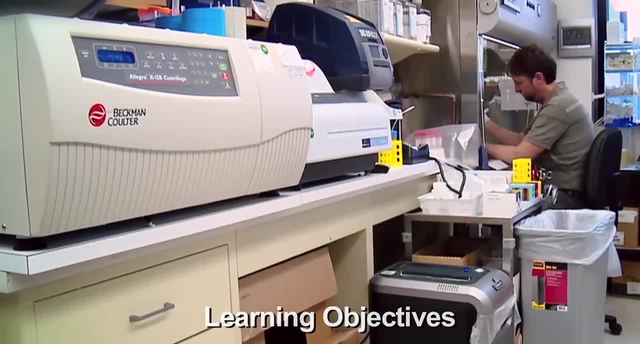 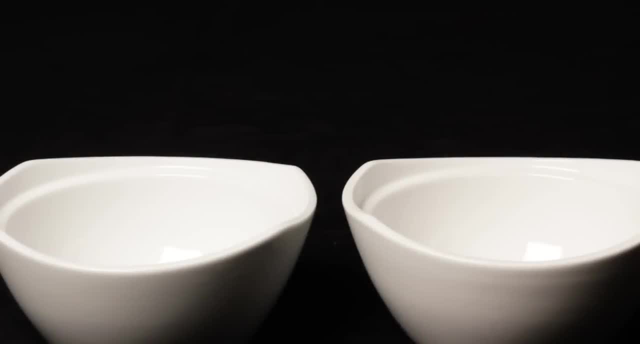 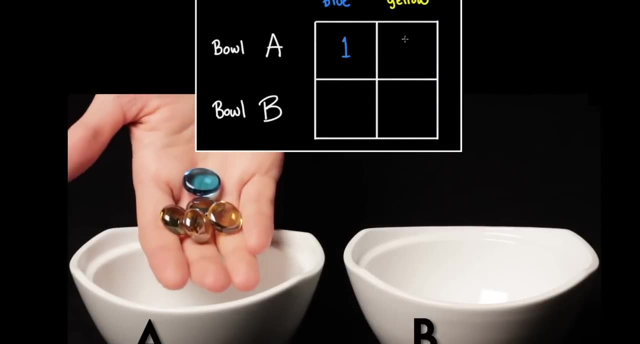 And understand how conditional probability can be used to interpret medical diagnoses. Suppose that in front of you are two bowls labeled A and B. Each bowl contains 5 marbles. Bowl A has 1 blue and 4 yellow marbles. Bowl B has 3 blue and 2 yellow marbles. 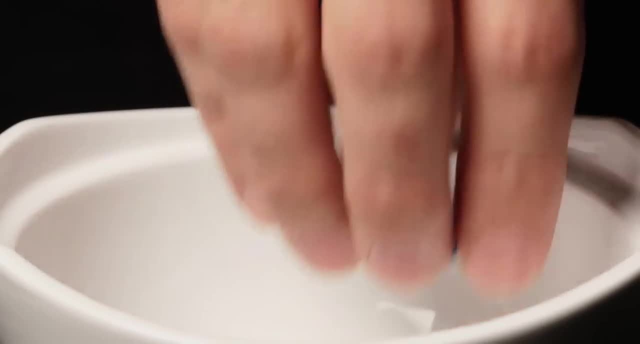 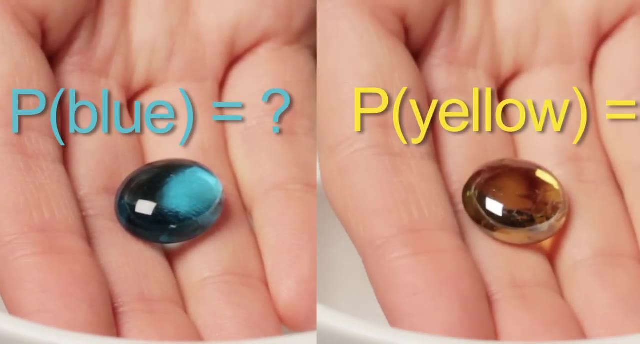 Now choose a bowl at random and draw a marble uniformly at random from it. Based on your existing knowledge of probability, of probability, how likely is it that you pick a blue marble? How about a yellow marble? Pause the video. When the number of possible outcomes is finite and all outcomes are equally likely, the probability- 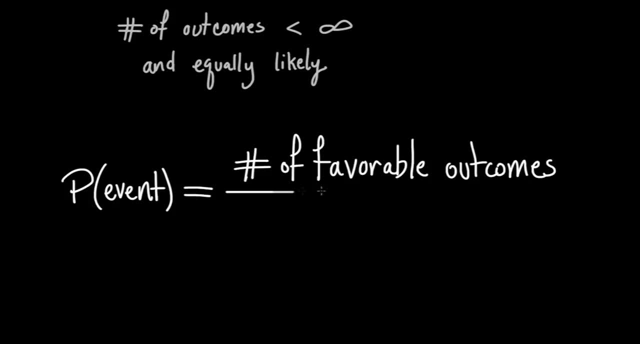 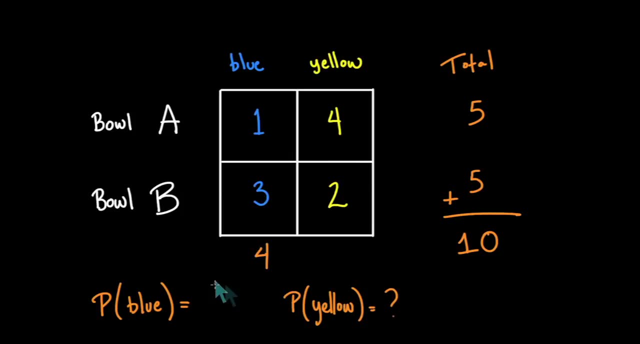 of an event happening is the number of favorable outcomes divided by the total number of possible outcomes. Out of the 10 marbles you could choose from, four are blue, so the probability of choosing a blue marble is four out of ten. There are six yellow marbles out of ten total. 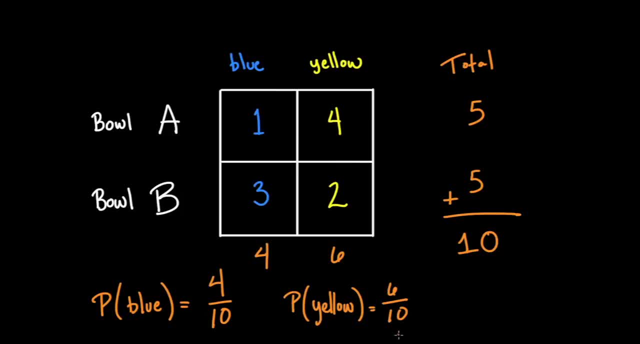 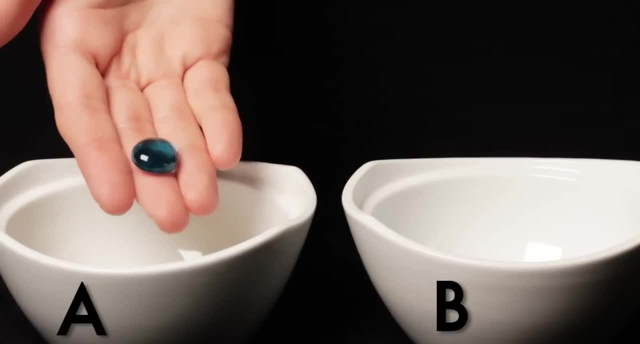 so the probability of choosing yellow is six out of ten. What if you must draw from bowl A? What's the probability of drawing a blue marble, given that you draw from bowl A? Pause the video. Let's go to the next slide. 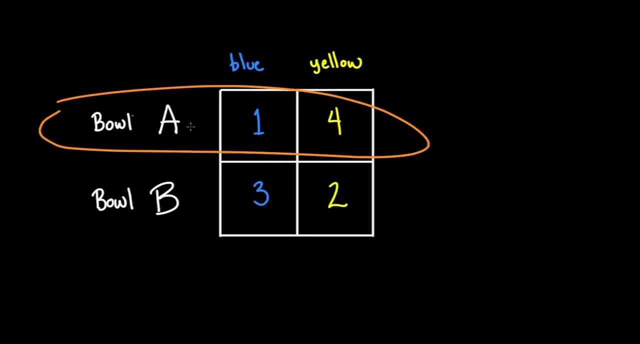 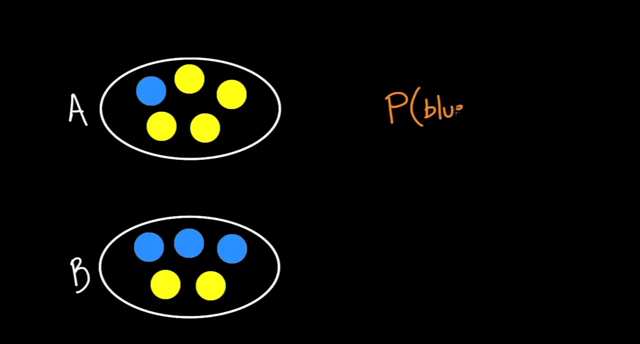 Let's go back to the table and consider only bowl A. Bowl A contains 5 marbles, of which one is blue. so the probability of picking a blue one is 1 in 5.. Notice that the probability has changed. In the first scenario, the sample space consists of all 10 marbles, because we are free to 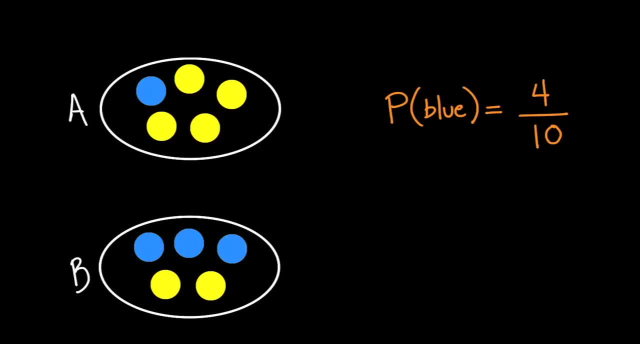 draw from both bowls. In the second scenario we are restricted to bowl A. Our new sample space consists of only the 5 marbles in bowl A. We ignore the marbles in bowl B. Restricting our attention to a specific set of outcomes changes the sample space and can. 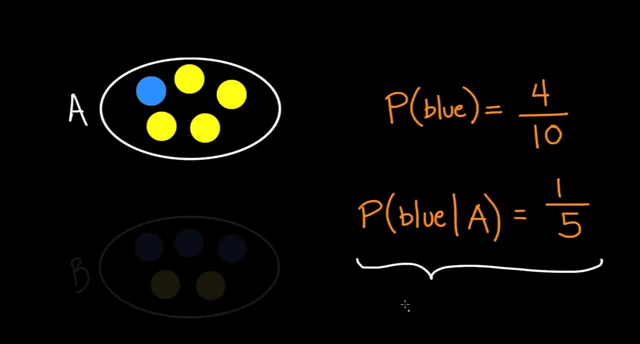 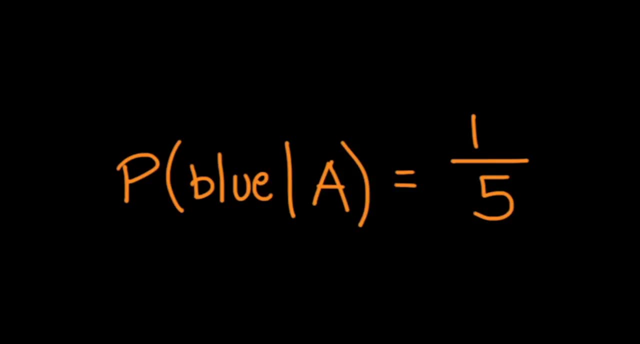 also change the probability of an event. This new probability is what we call a conditional probability. This is standard notation for conditional probability. The vertical bar is read as given: The probability we are looking for precedes the bar and the condition follows the bar. 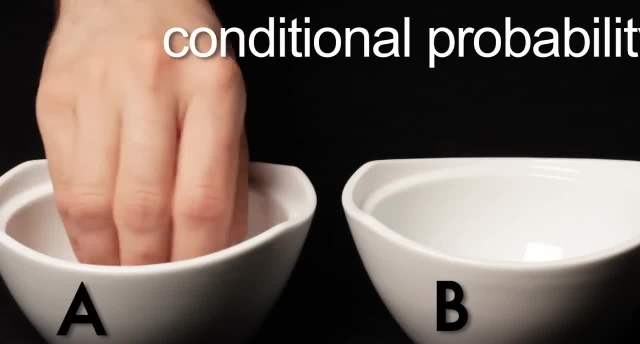 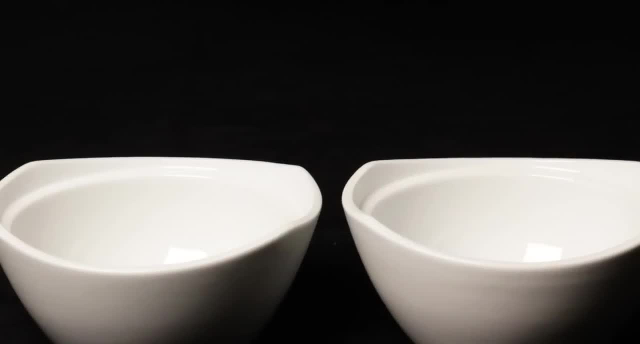 In the previous example we calculated the conditional probability of drawing a blue marble, given that we draw from bowl A. Now let's flip things around. Suppose someone picks a marble at random from either bowl A or bowl B and reveals to you that the marble drawn was blue. 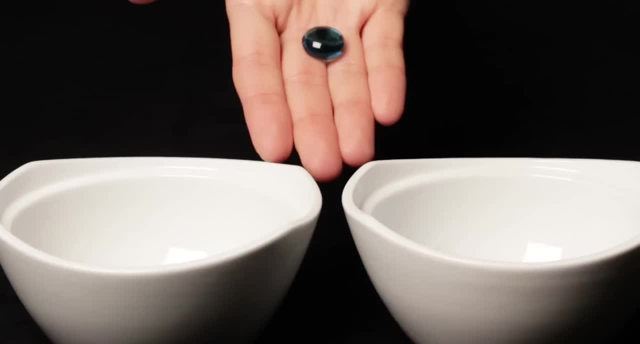 What is the probability that the blue marble came from bowl B? The answer is A. In other words, what is the conditional probability that the marble was drawn from bowl A, given that it is blue? Pause the video and try to work this out. 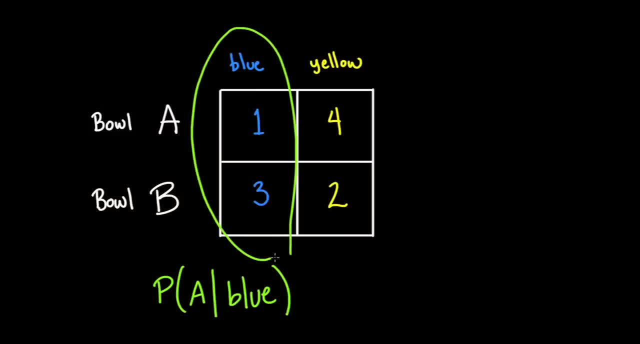 Going back to the table, because we are dealing with the condition that the marble is blue. the sample space is restricted to the 4 blue marbles. Of these 4 blue marbles, one is in bowl A. Each is also in bowl B. 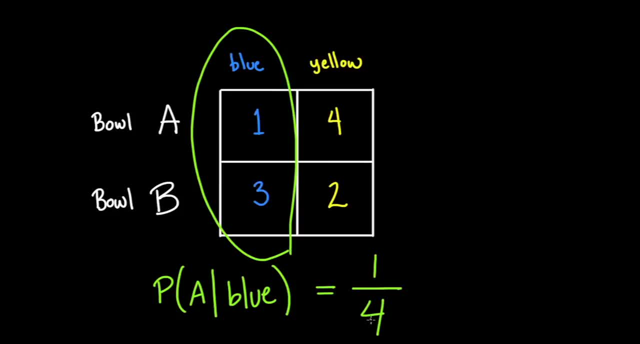 The next table is in bowl A and each is equally likely to be drawn. Thus, the conditional probability is 1 out of 4.. Notice that the probability of picking a blue marble, given that the marble came from bowl A, is NOT equal to the probability that the marble came from bowl A, given that the marble 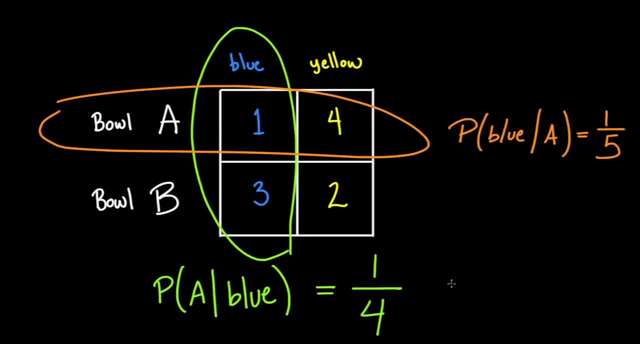 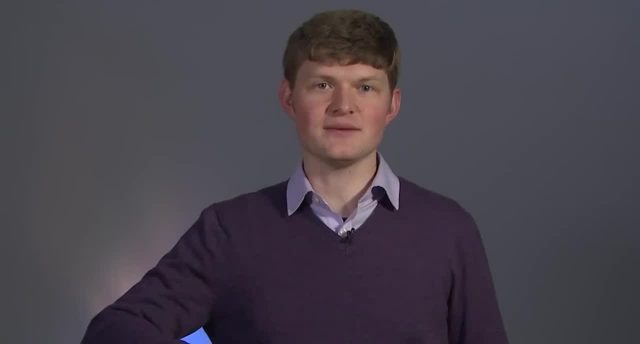 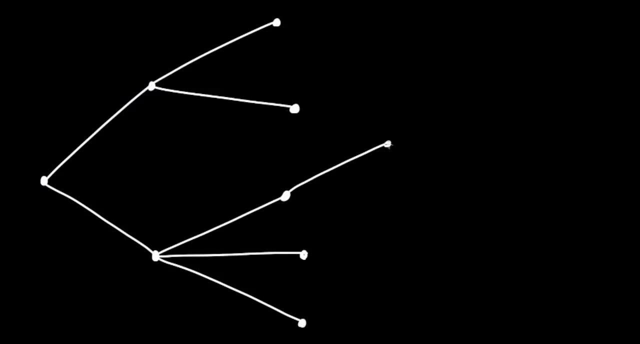 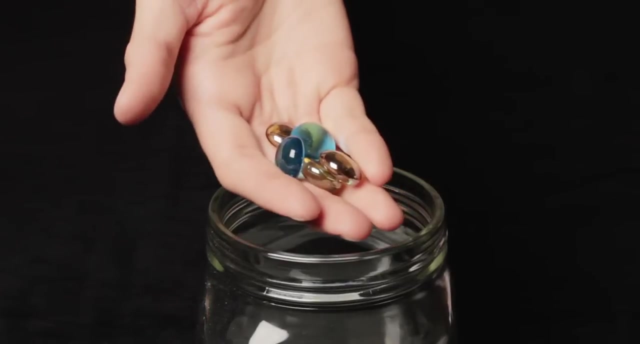 was blue. Each has a different condition, so be careful not to mix them up. organize our data and visualize changes in the sample space. Let's look at another tool that is useful for understanding conditional probabilities: a tree diagram. Suppose we have a jar containing five marbles: Two are blue and 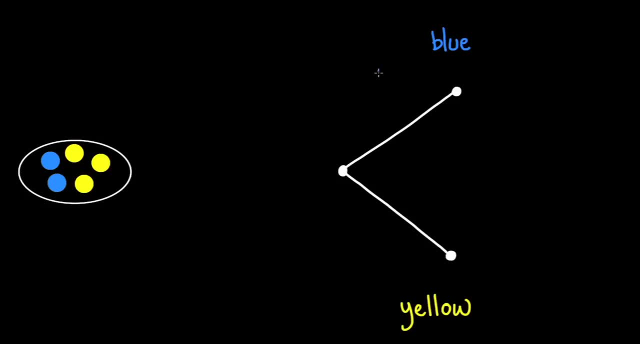 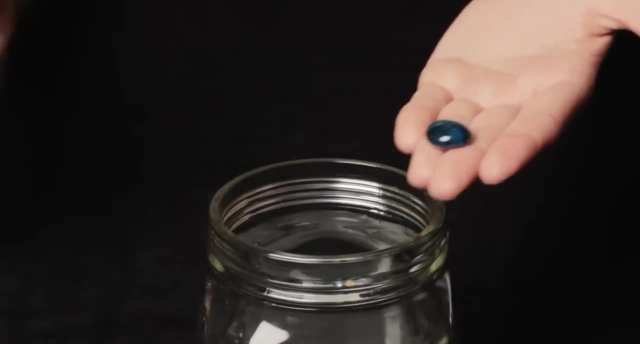 three are yellow. If we draw any one marble at random, the probability of drawing a blue marble is two-fifths. Now, without replacing the first marble, draw a second marble from the jar. Given that the first marble is blue, is the. 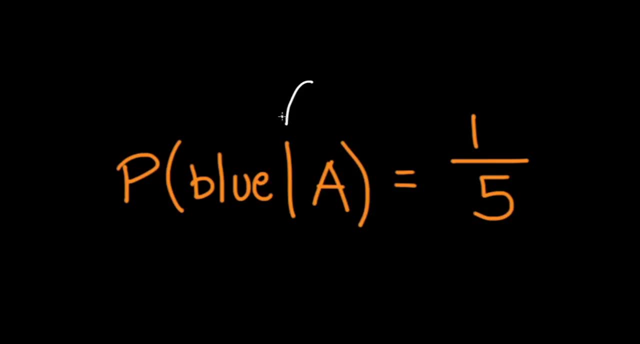 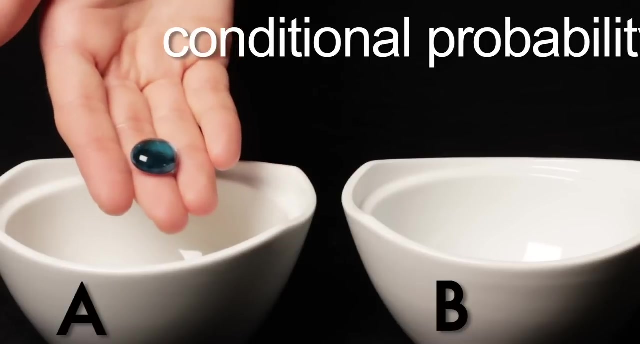 standard notation for conditional probability. The vertical bar is read as given: The probability we are looking for precedes the number of marbles. The number of marbles in bowl A is precedes the bar and the condition follows the bar. In the previous example we calculated the conditional probability of drawing a blue. 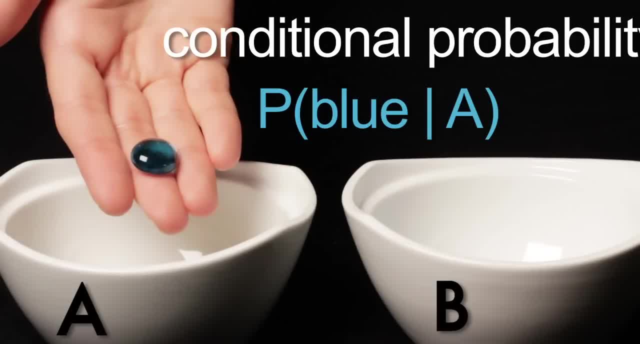 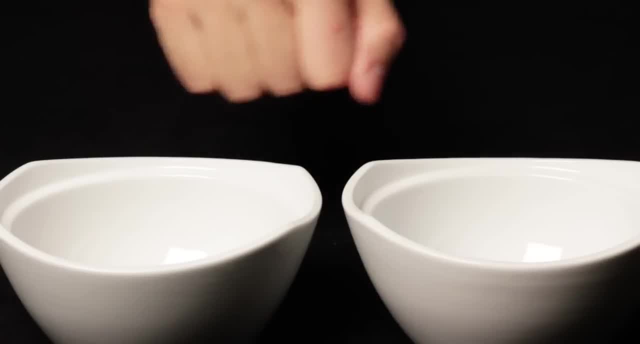 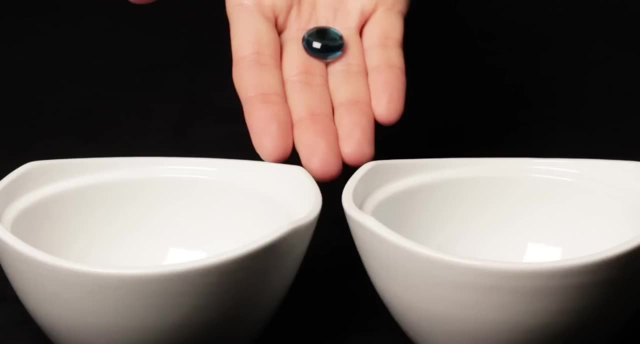 marble, given that we draw from bowl A. Now let's flip things around. Suppose someone picks a marble at random from either bowl A or bowl B and reveals to you that the marble drawn was blue, What is the probability that the blue marble came from bowl A? In other, 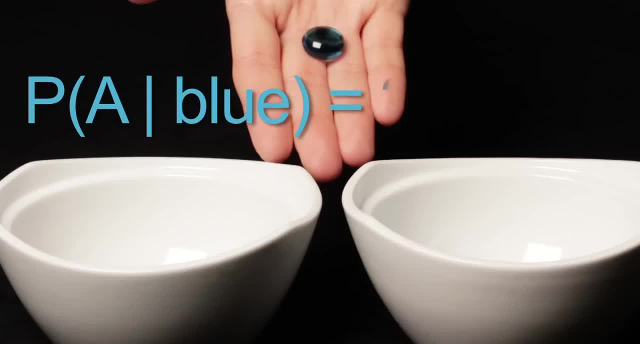 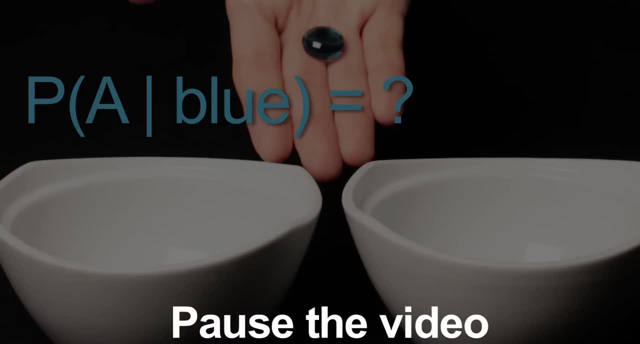 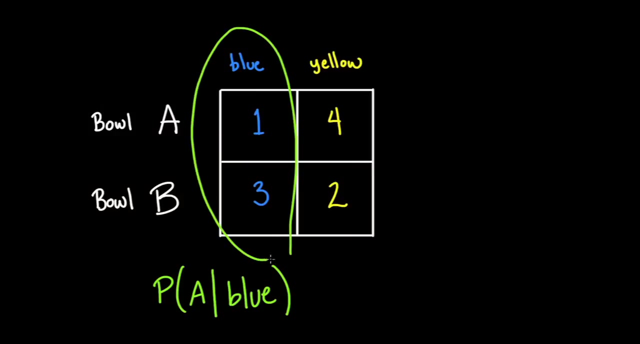 words. what's the conditional probability that the marble was drawn from bowl A, given that it is blue? Pause the video and try to work this out. Going back to the table, because we are dealing with the condition that the marble is blue, the sample space is restricted to the four blue marbles. Of these four blue marbles, 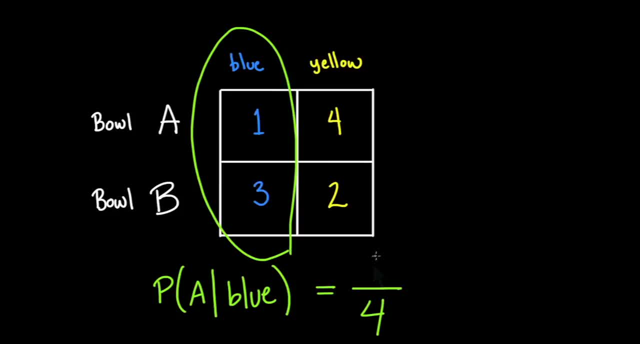 one is in bowl A and each is equally likely to be drawn Subtitles by the Amaraorg community. Thus, the conditional probability is one out of four. Notice that the probability of picking a blue marble, given that the marble came from bowl A, is not equal to the probability that the marble came from bowl A, given that the marble 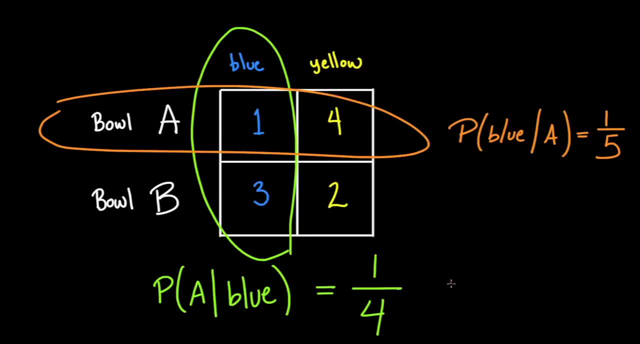 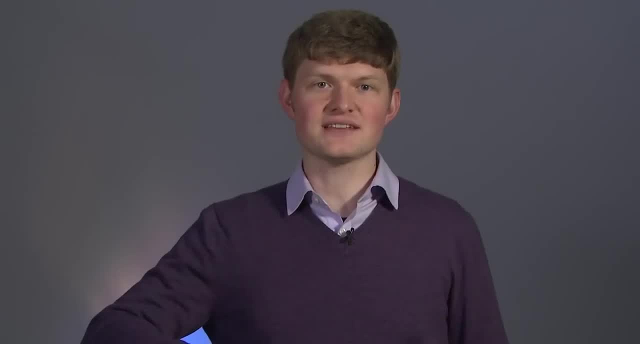 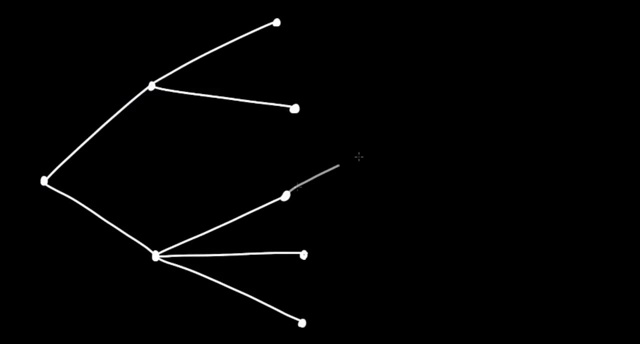 was blue. Each has a different condition, so be careful not to mix them up. We've seen how tables can help us organize our data and visualize changes in the table In the sample space. let's look at another tool that is useful for understanding conditional. 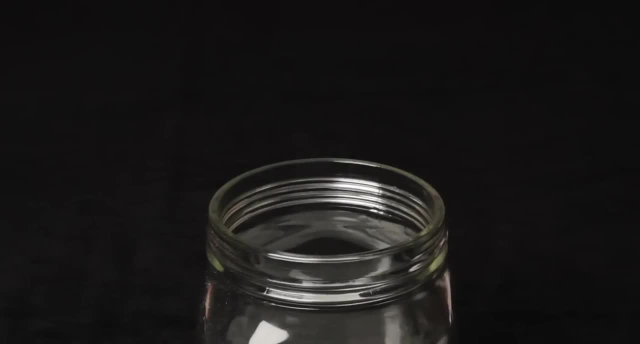 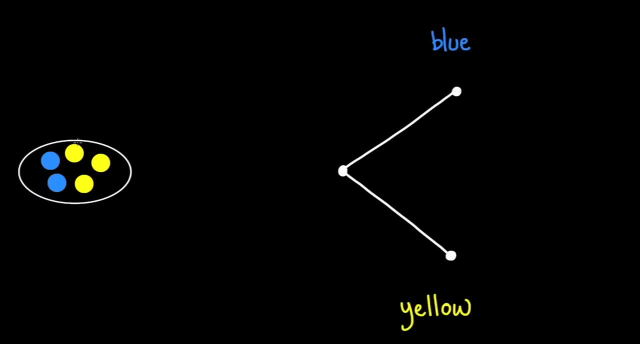 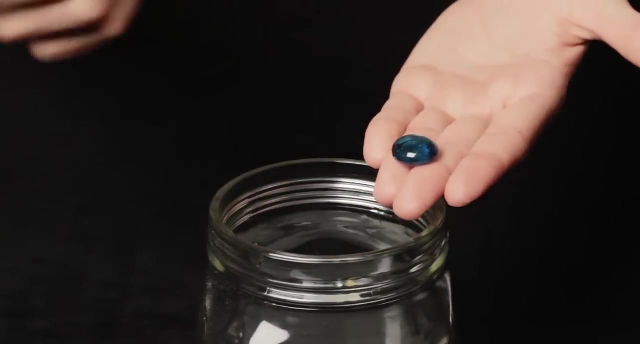 probabilities, a tree diagram. Suppose we have a jar containing five marbles. Two are blue and three are yellow. If we draw any one marble at random, the probability of drawing a blue marble is two fifths. Now, without replacing the first marble, draw a second. 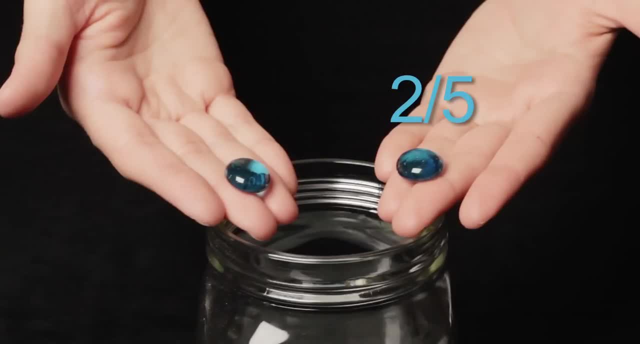 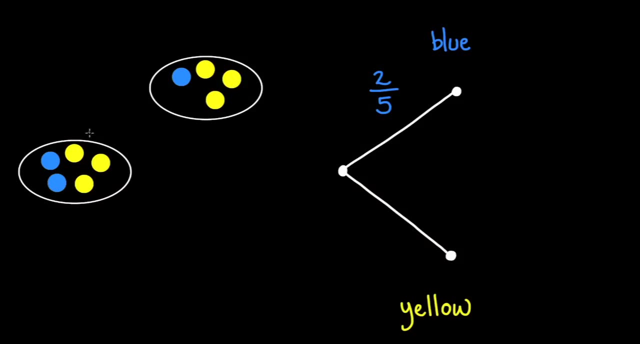 marble from the jar. Given that the first marble is blue, is the probability of drawing a second blue marble still two fifths? No, it isn't. Our sample space has changed. If a blue marble is drawn first, you are left with four marbles: one blue and three yellow. 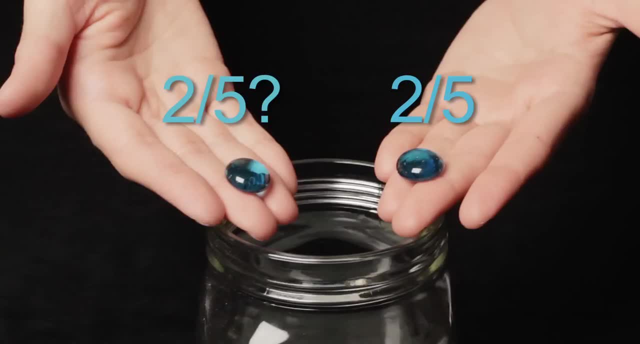 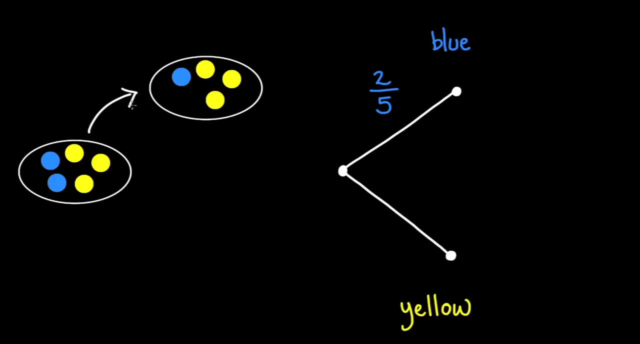 probability of drawing a second blue marble still two-fifths. No, it isn't. Our sample space has changed. If a blue marble is drawn first, you're left with four marbles: one blue and three yellow. In other words, if a blue marble is, 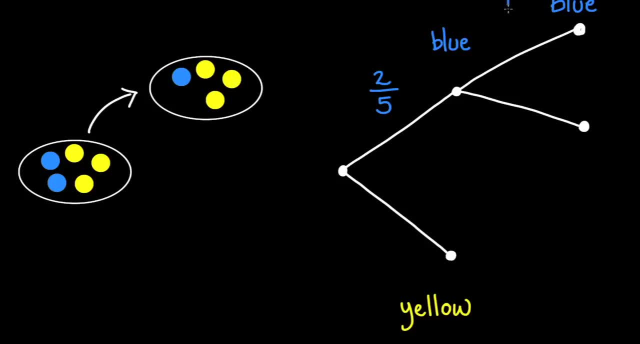 selected first, the probability that you draw a blue second is one-fourth and the probability that you draw a yellow second is three-fourths. you Now pause the video and determine the probabilities if the yellow marble is selected first. instead, If a yellow marble is selected first, you are left with two yellow and two blue. 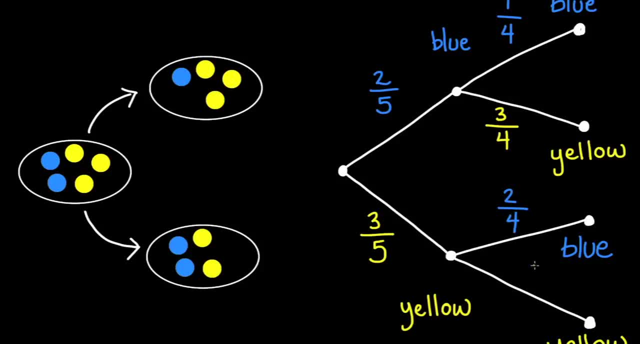 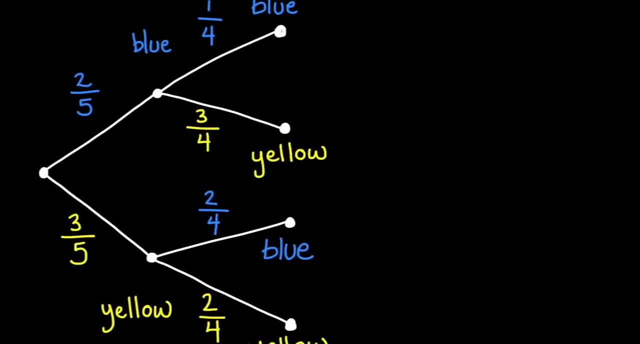 marbles. There is now a two-fourths chance of drawing a blue marble and a two-fourths chance of drawing a yellow marble. What we have drawn here is called a tree diagram. Tree diagrams help us to visualize our sample space and reason out probabilities. 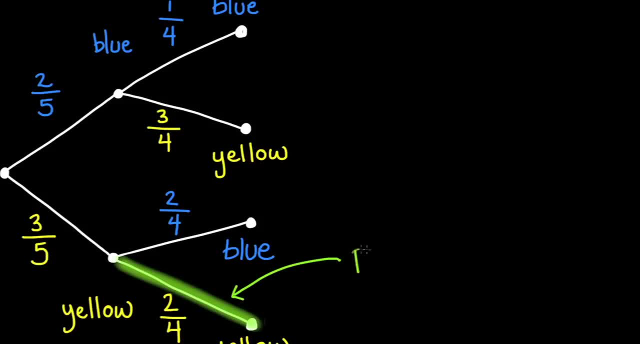 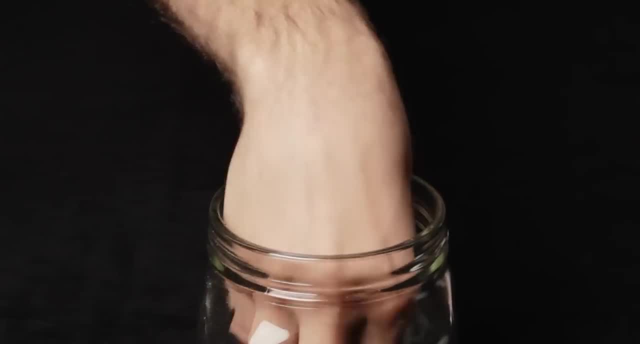 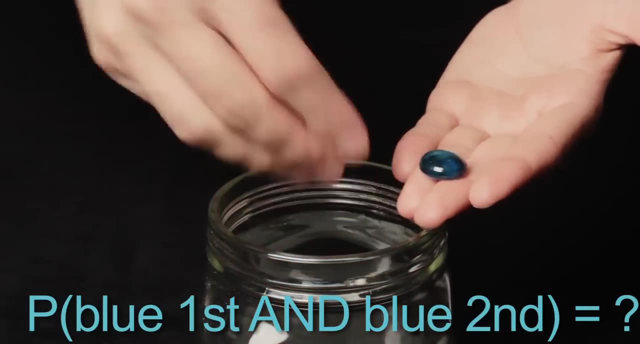 The probability assigned to the second branch denotes the conditional probability. given that the first happened, We can answer questions like: what is the probability of drawing two blue marbles in a row? In other words, what is the probability of drawing a blue marble first and a blue marble second? 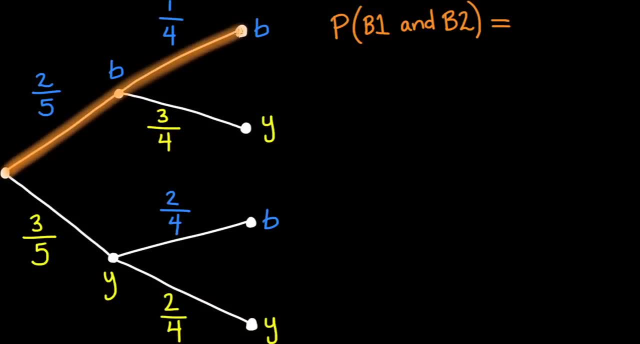 This event is represented by these two branches in the tree diagram. We have a two-fifths chance, which applies to drawing two marbles. 或 This event is represented by these two branches in the tree diagram chance, followed by a one-fourth chance. We multiply these to get two-twentieths or one-tenth. 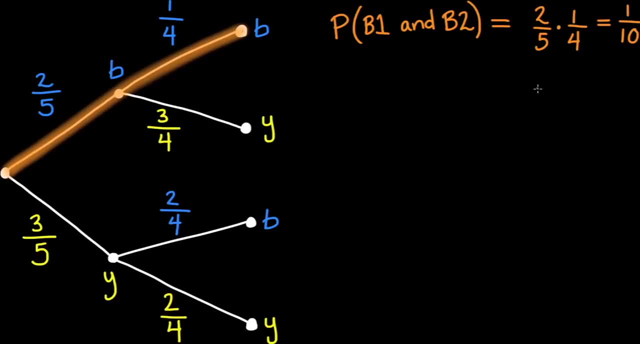 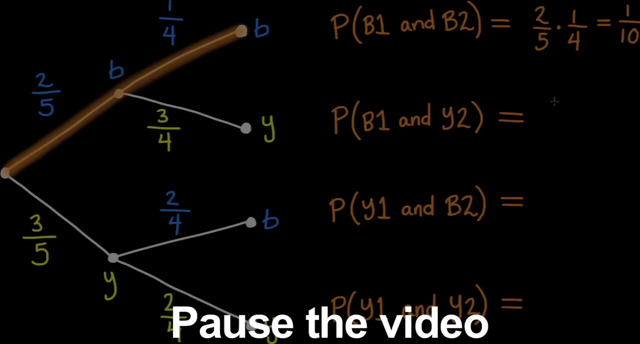 The probability of drawing two blue marbles in a row is one-tenth. Now you do it. Use the tree diagram to calculate the probabilities of the other possibilities – blue-yellow, yellow-blue and yellow-yellow. The probabilities each work out to three-tenths. The four probabilities add up to a total of 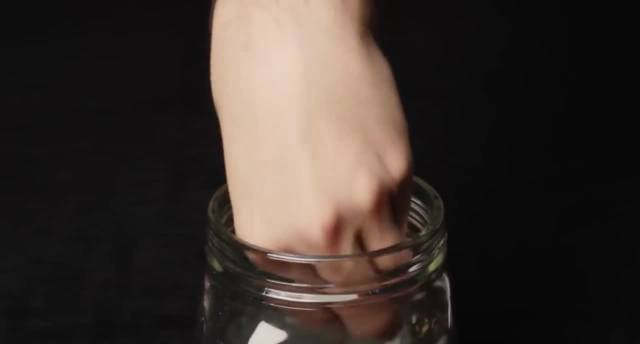 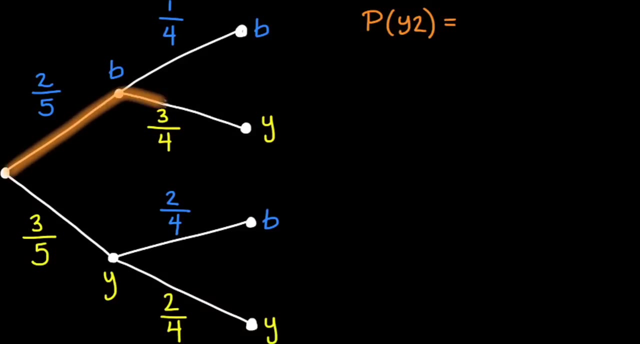 one, as they should. What if we don't care about the first marble? We just want to determine the probability that the second marble is yellow, Because it does not matter whether the first marble is blue or yellow. we consider both: the blue-yellow and yellow-yellow paths. 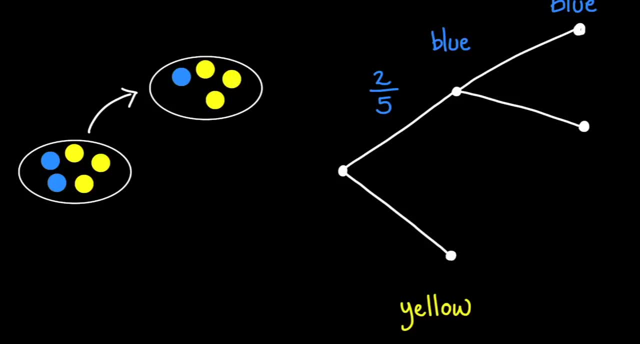 In other words, if a blue marble is selected first, the probability that you draw a blue second is one fourth and the probability that you draw a yellow second is three fourths. Now pause the video and determine the probabilities if the yellow marble is selected first. 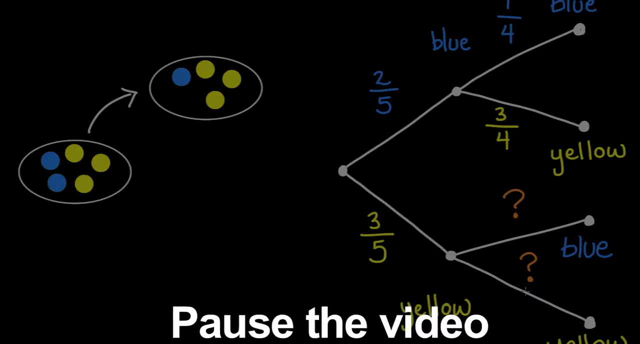 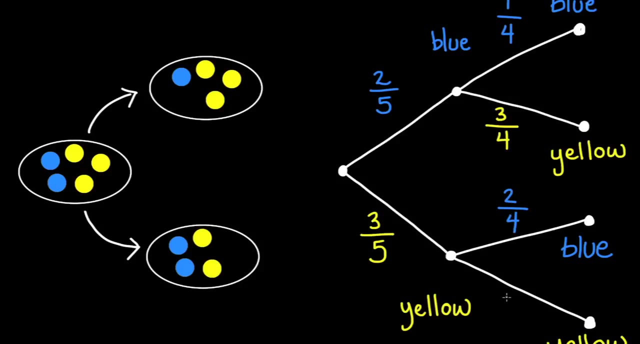 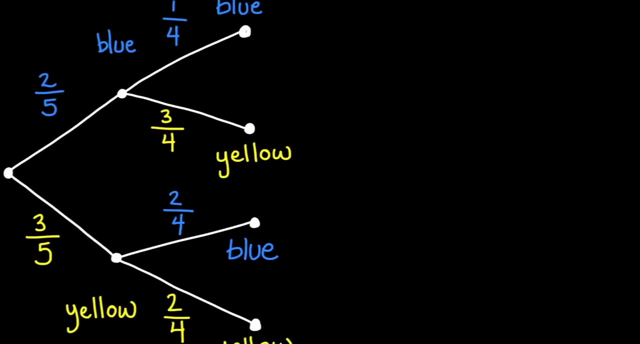 Subtitles by the Amaraorg community. If a yellow marble is selected first, you are left with two yellow and two blue marbles. There is now a two fourths chance of drawing a blue marble and a two fourths chance of drawing a yellow marble. What we have drawn here is called a tree diagram. 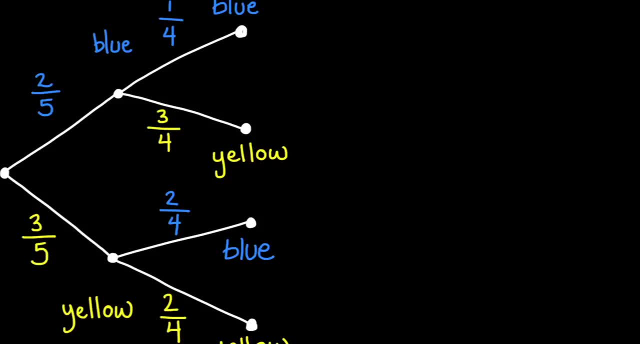 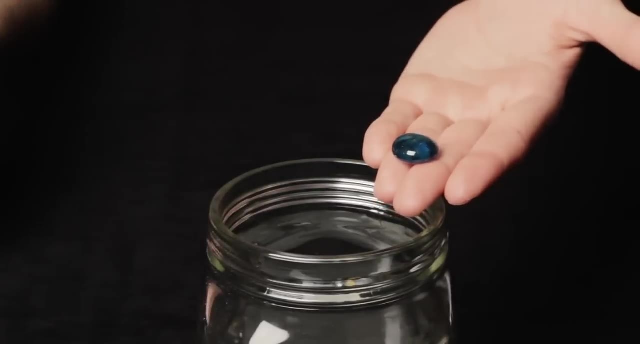 Tree diagrams help us to visualize our sample space and reason out probabilities. The probability assigned to the second branch denotes the conditional probability, given that the first happened. We can answer questions like: What is the probability of drawing two blue marbles in a row? In other words, what is the probability of drawing a blue marble first and a blue? 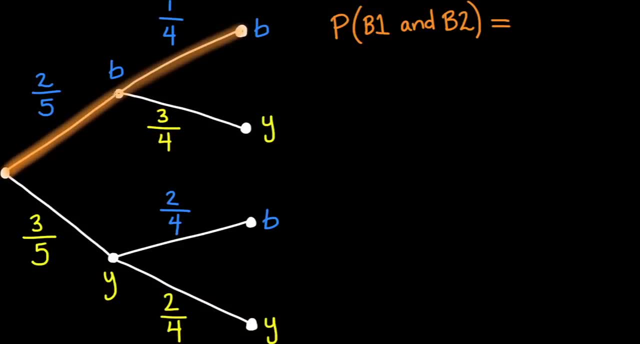 marble second. This event is represented by these two branches in the tree diagram. We have a two fifths chance, followed by a one fourth chance. We multiply these to get two twentths or one tenths. Subtitles by the Amaraorg community. 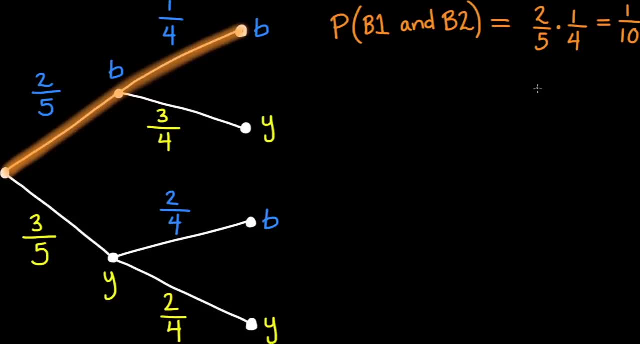 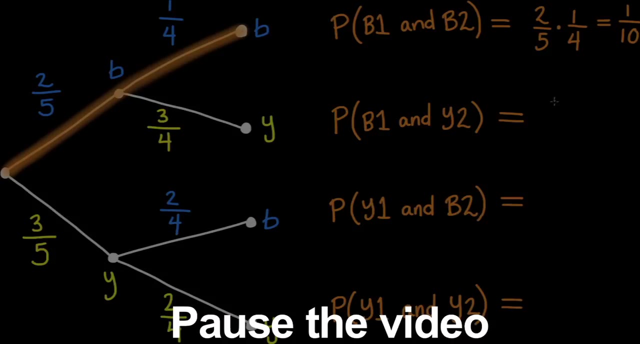 The probability of drawing two blue marbles in a row is one-tenth. Now you do it. Use the tree diagram to calculate the probabilities of the other possibilities: blue-yellow, yellow-blue and yellow-yellow. The probabilities each work out to three-tenths. 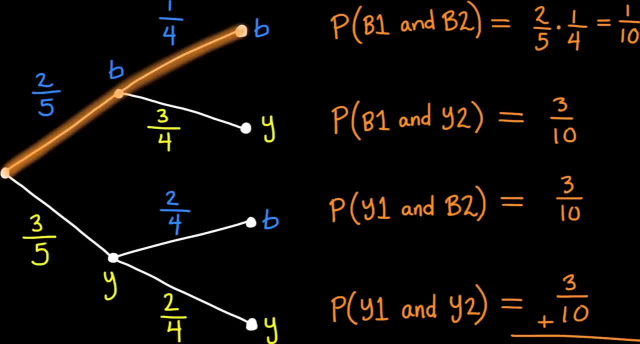 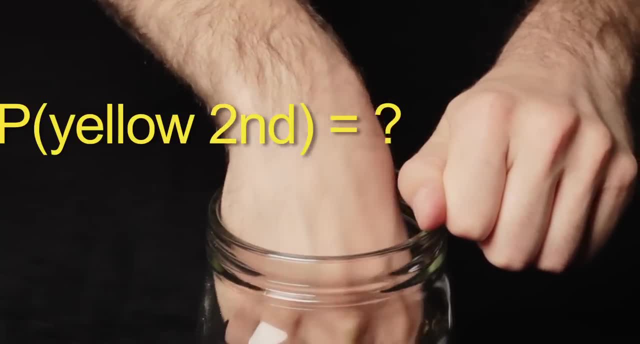 The four probabilities add up to a total of one, as they should. What if we don't care about the first marble? We just want to determine the probability that the second marble is yellow, Because it does not matter whether the first marble is blue or yellow. 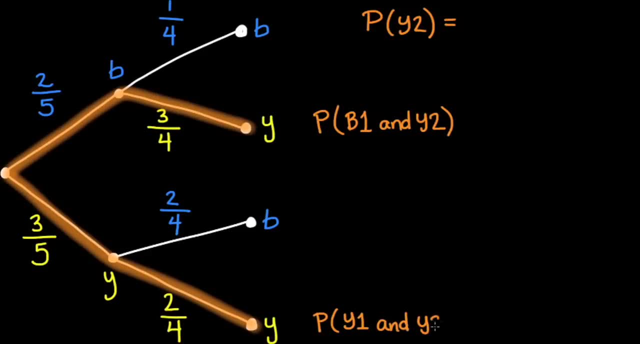 we consider both the blue-yellow and yellow-yellow paths. Adding the probabilities gives us three-tenths plus three-tenths, which works out to three-fifths. Here's another interesting question: What is the probability that the first marble drawn is blue? 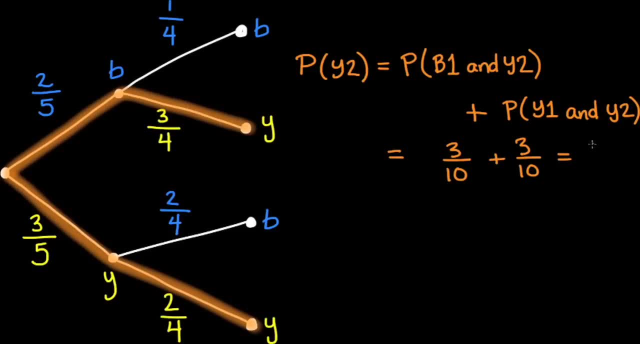 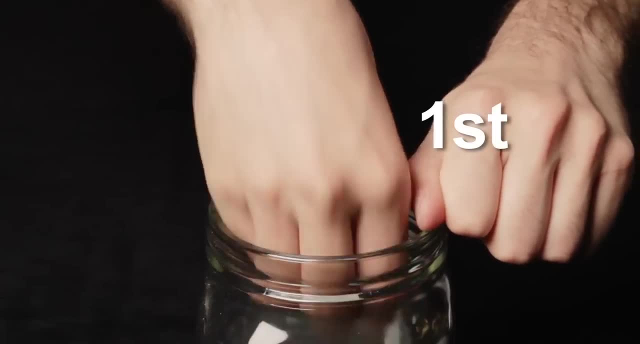 Adding the probabilities gives us three-tenths plus three-tenths, which works out to three-fifths. Here's another interesting question: What is the probability that the first marble drawn is blue, given that the second marble drawn is yellow? 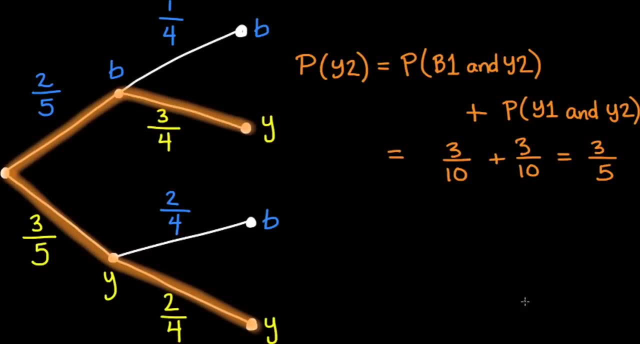 Intuitively. this seems tricky. Pause the video and reason through the probability tree with a friend, Because we are conditioning on the event that the second marble drawn is yellow. our sample is yellow, So the sample space is restricted to these two paths. 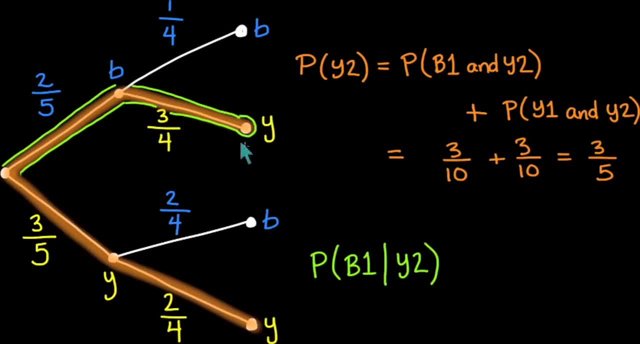 Of these two paths, only the top one meets our criterion – that the blue marble is drawn first. We represent the probability as a fraction of favorable to possible outcomes. Hence the probability that the first marble drawn is blue, given that the second marble drawn 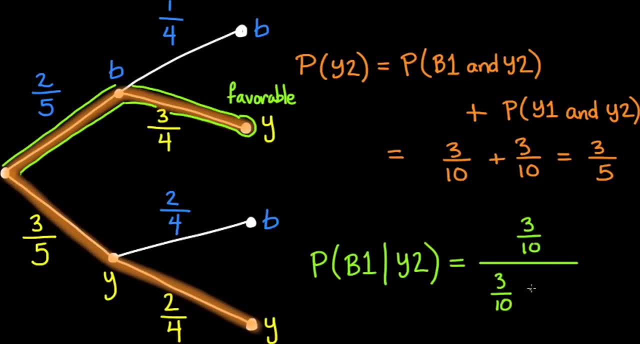 is yellow is three-tenths divided by three-tenths plus three-tenths, which works out to one-half. I hope you appreciate that this information is useful. Please let us know in the comments. I'd love to hear from you about the sample space. 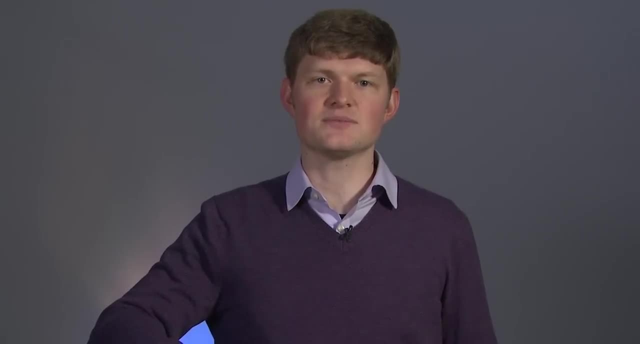 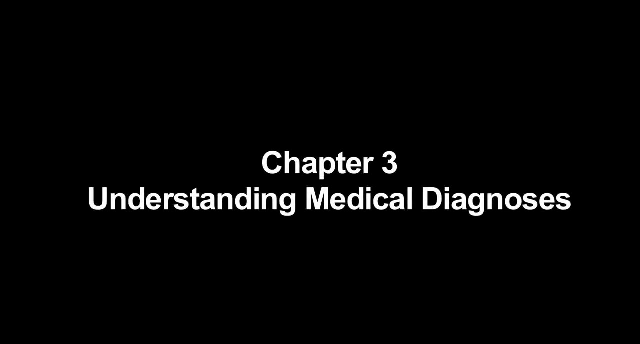 Thank you. Thank you, I'm Daniel Vosler. I'll see you next time, Bye-bye, Bye-bye, Bye-bye. tree diagrams and tables make these types of probability problems doable without having to memorize any formulas. 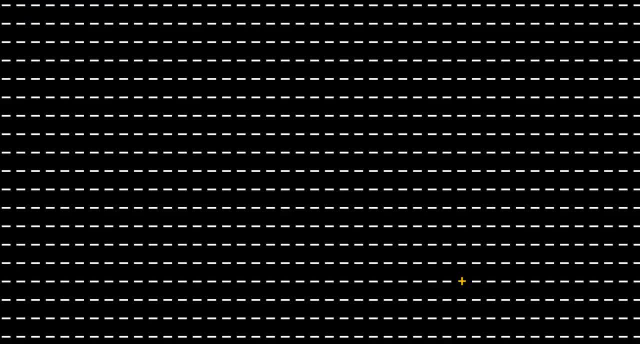 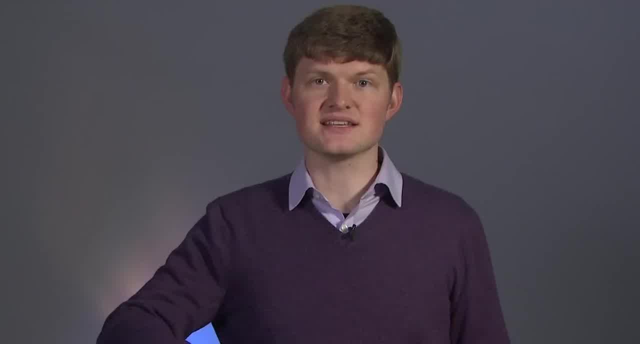 Let's return to our opening question. Recall that you've tested positive for a cancer that afflicts 1 out of 1000 people, based on a test that is 99% accurate. More precisely, out of 100 test results, we expect about 99 correct results and only 1 incorrect result, Since 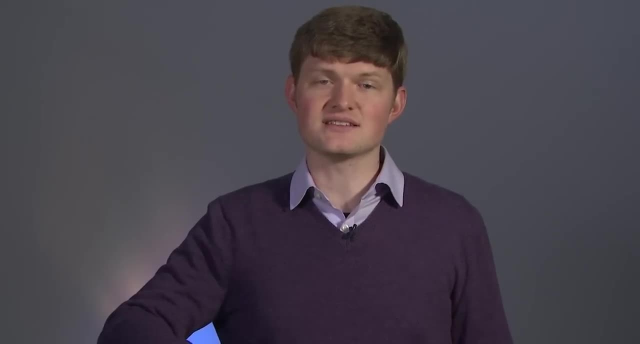 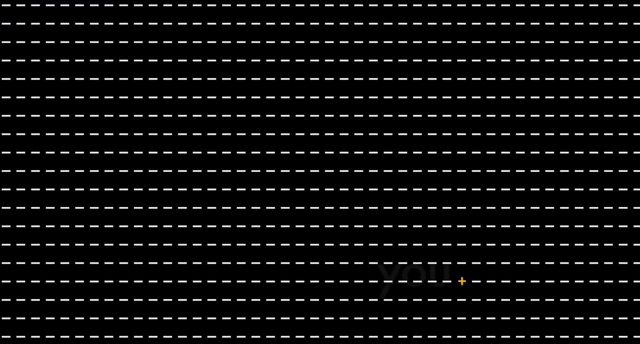 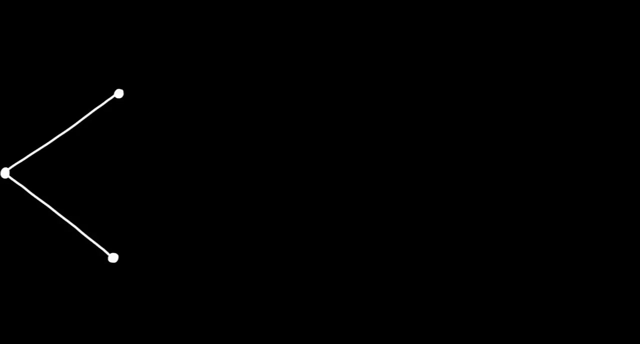 the test is highly accurate. you might conclude that the test is unlikely to be wrong and that you most likely have cancer. But wait. Let's first use conditional probability to make sense of our seemingly gloomy diagnosis. Let's use a tree diagram to help with our calculations. The first branch of the tree. 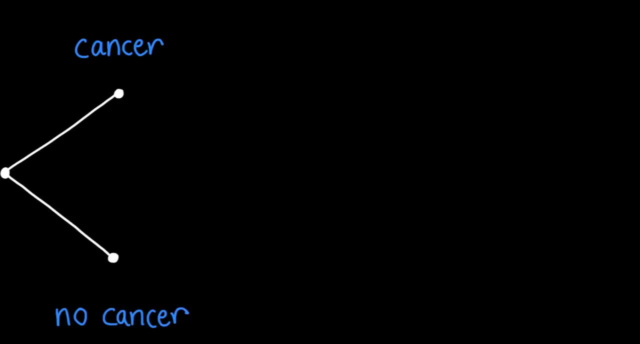 represents the likelihood of cancer in the general population. The probability of having the cancer is 1 in 1000, or .001.. The probability of having no cancer is .999.. Let's extend the tree diagram to illustrate the possible results of the medical test that. 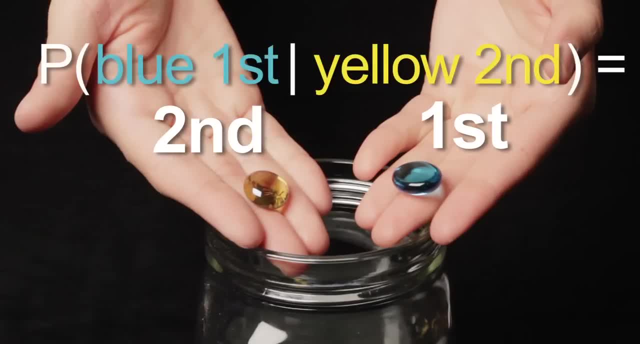 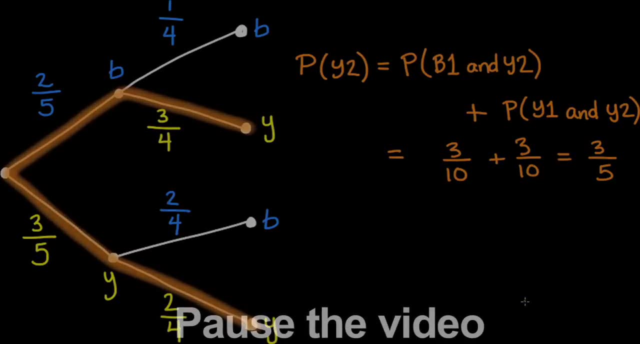 given that the second marble drawn is yellow, Intuitively this seems tricky. Pause the video and reason through the probability tree with a friend. Because we are conditioning on the event that the second marble drawn is yellow, our sample space is restricted to these two paths. 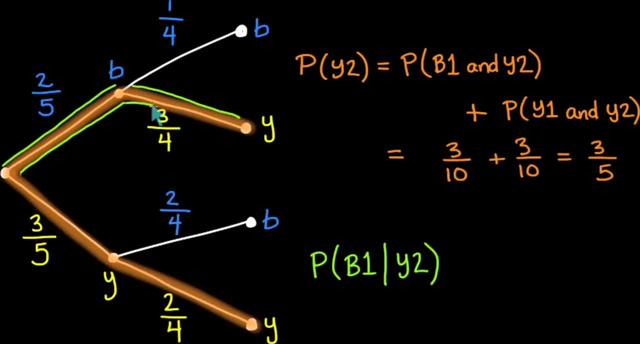 Of these two paths, only the top one meets our criteria. So the probability that the first marble drawn is yellow is three-tenths, and the probability that the second marble drawn is yellow is three-tenths. We represent the probability as a fraction of favorable to possible outcomes. 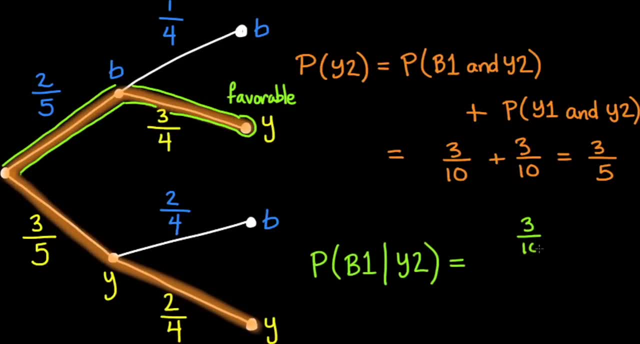 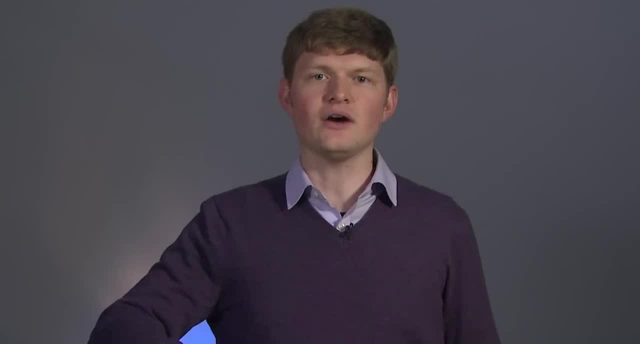 Hence the probability that the first marble drawn is blue, given that the second marble drawn is yellow, is three-tenths divided by three-tenths plus three-tenths, which works out to one-half. I hope you appreciate that. tree diagrams and tables. 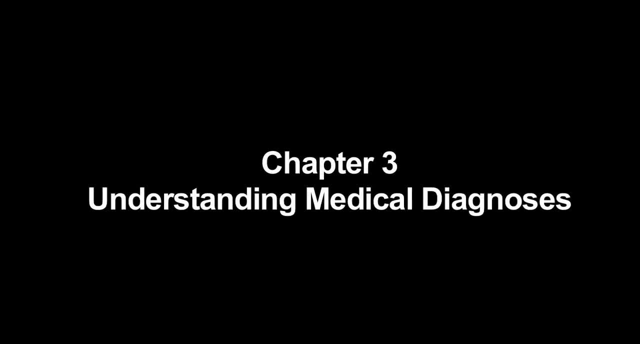 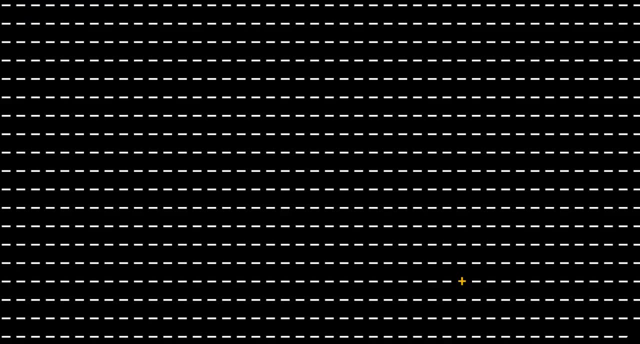 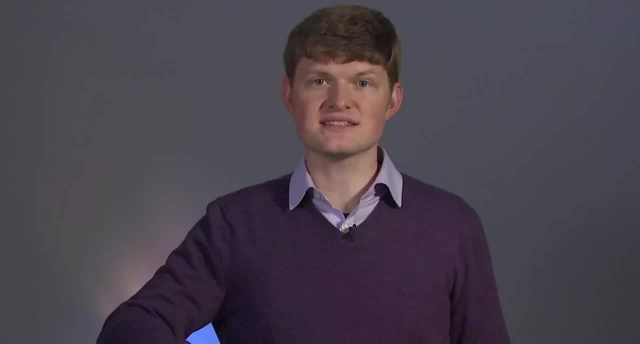 without having to memorize any formulas. Let's return to our opening question. Recall that you've tested positive for a cancer that afflicts one out of a thousand people, based on a test that is 99% accurate. More precisely, out of 100 test results. 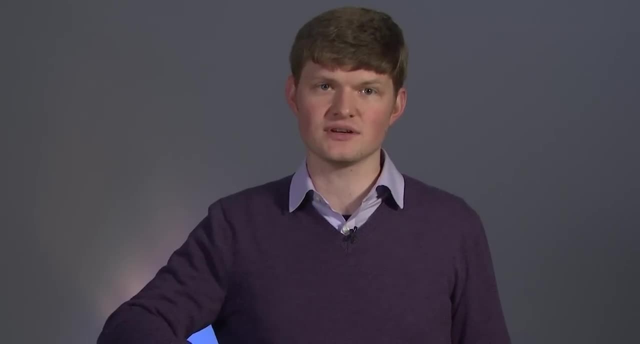 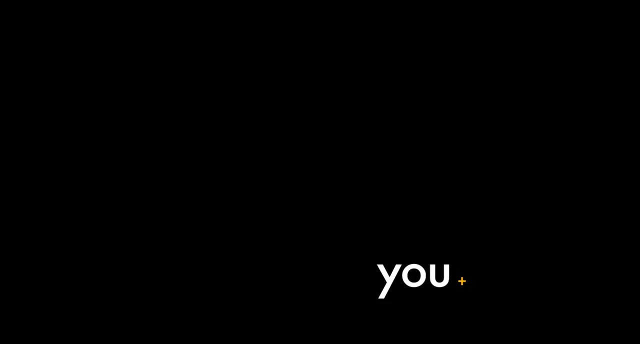 we expect about 99 correct results and only one incorrect result. Since the test is highly accurate, you might conclude that the test is unlikely to be wrong and that you most likely have cancer. But wait, Let's first use conditional probability to make sense of our seemingly gloomy diagnosis. 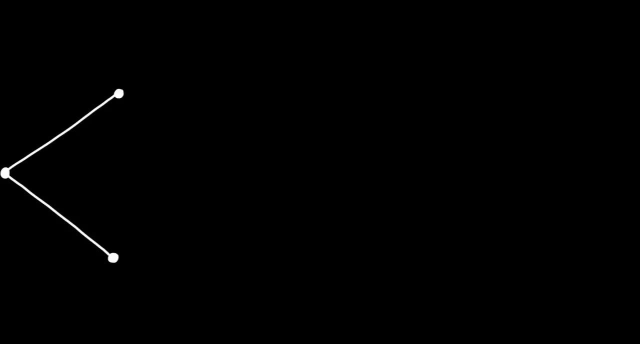 Let's use a tree diagram to help with our calculations. The first branch of the tree represents the likelihood of cancer in the general population. The probability of having the cancer is one in a thousand or .001.. The probability of having no cancer is .999.. 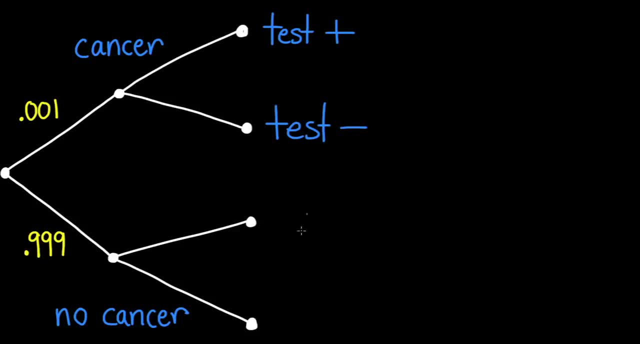 Let's extend the tree diagram to illustrate the possible results of the medical test. that is 99% accurate In the cancer population. 99% will test positive correctly, but 1% will test negative incorrectly. These incorrect results are called false negatives. 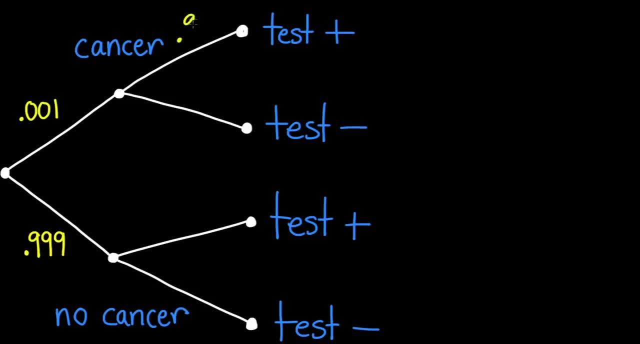 is 99% accurate. In the cancer-free population, 99% will test positive, but 1% will test negative incorrectly. These incorrect results are called false negatives. In the cancer-free population, 99% will test negative correctly correctly, but 1% will test positive incorrectly. These incorrect results are called false positives. 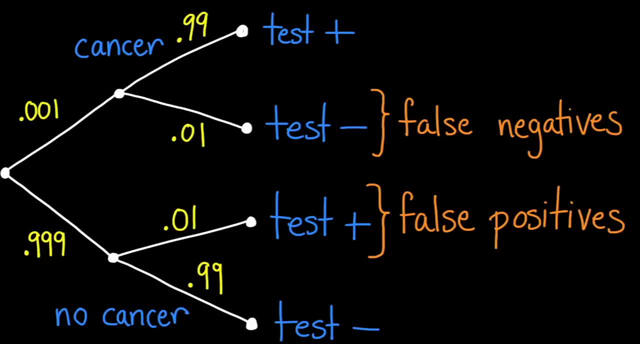 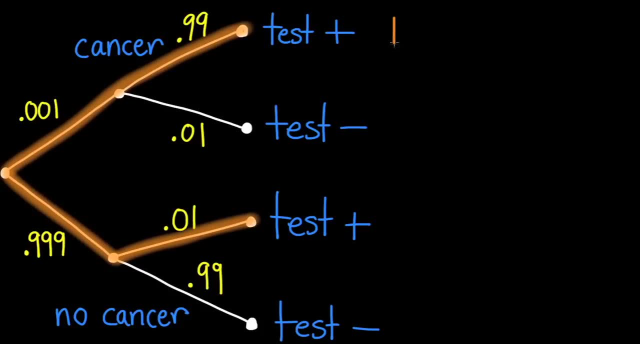 Given that you test positive, our sample space is now restricted to only the population that tested positive. This is represented by these two paths. The top path shows the probability you have the cancer and test positive. The lower path shows the probability you don't. 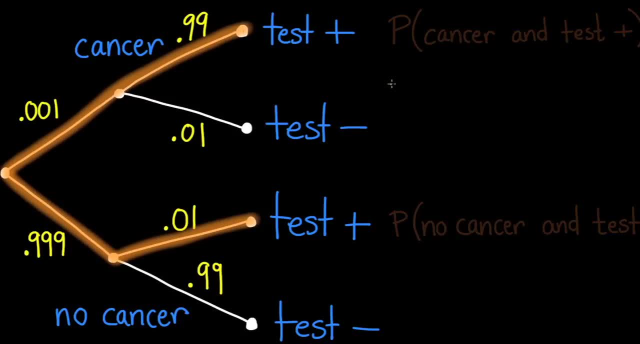 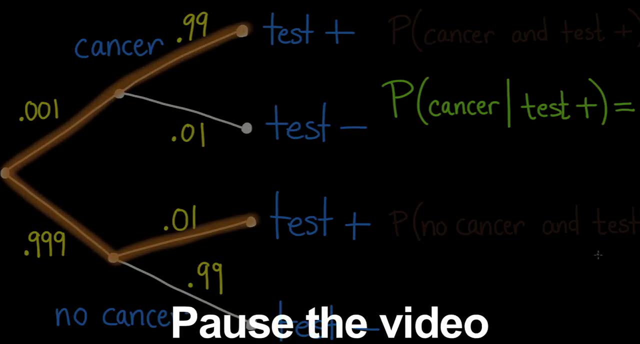 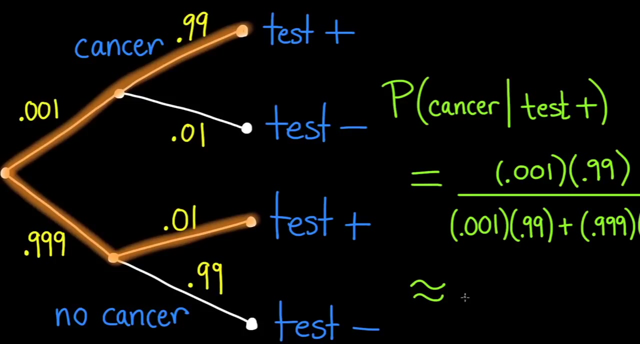 have the cancer and still test positive. Now pause the video and determine the probability that you have the cancer, given that you test positive. The probability that you actually do have the cancer, given that you test positive, is given by the following expression, which works out to about .09, less than 10%: The. 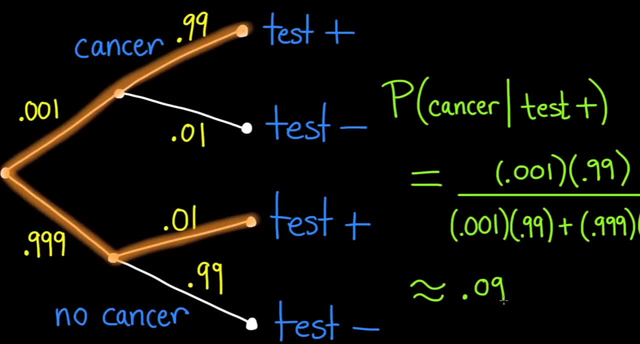 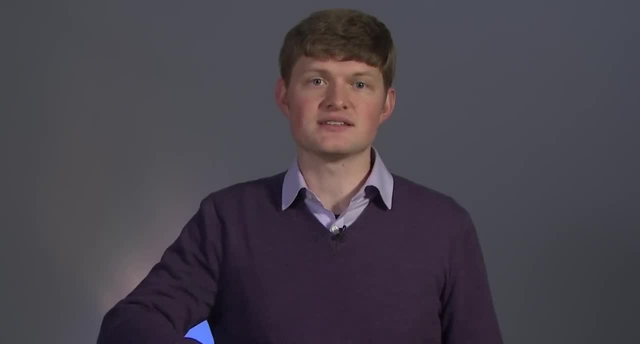 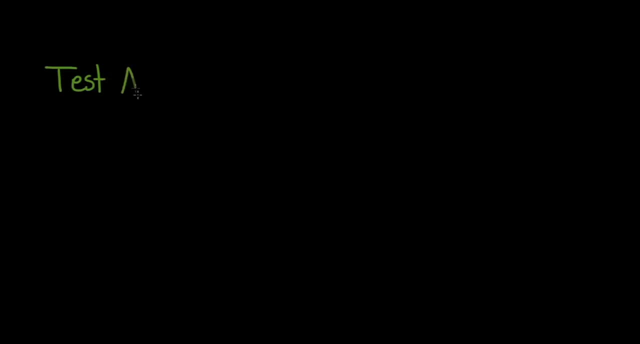 error rate of the test is only 1%, but the chance of a misdiagnosis is more than 90%. Chances are pretty good that you do not actually have the cancer, despite the rather accurate test. Why is this so? The accuracy of the test actually reflects the conditional probability that one tests. 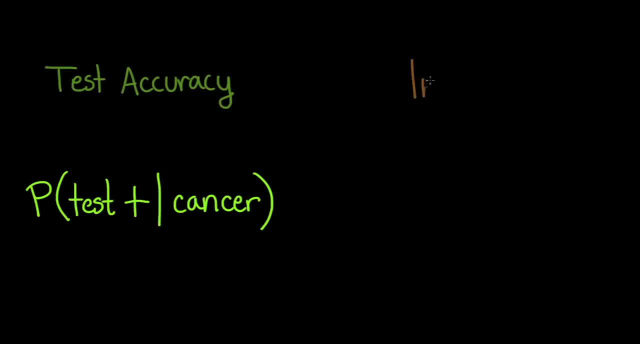 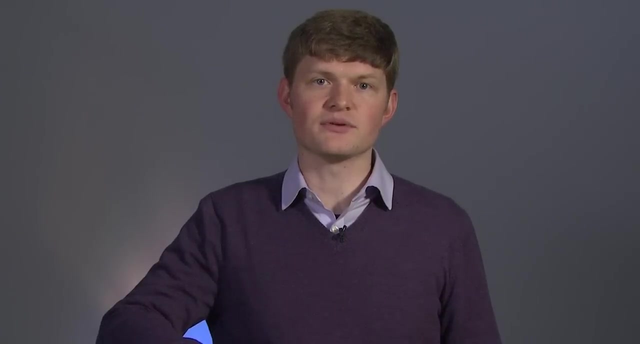 positive, given that one has cancer. But in practice, what you want to know is the conditional probability that you have cancer, given that you test positive. These probabilities are not the same. Whenever we take medical tests or perform experiments, it is important to understand what events our results are conditioned on and how that. 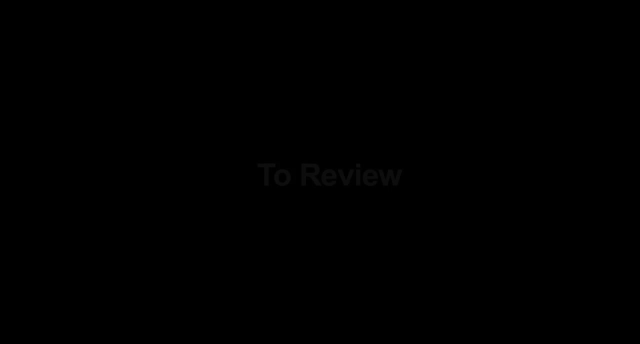 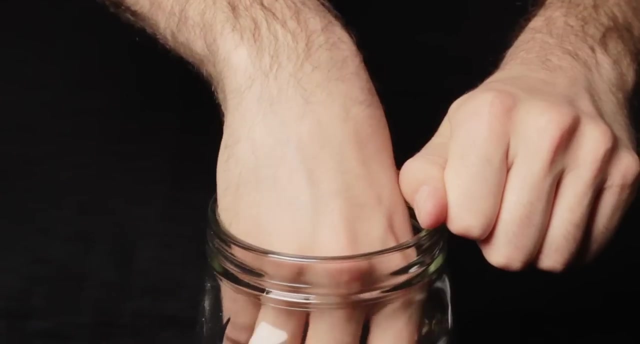 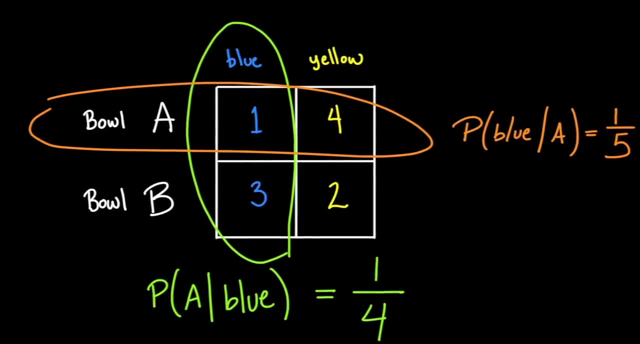 might affect the accuracy of our conclusions. In this video, you've seen that conditional probability must be used to understand and predict the outcomes of many events. You've also learned to evaluate and manage conditional probabilities using tables and trees. We hope that you will now think more carefully. 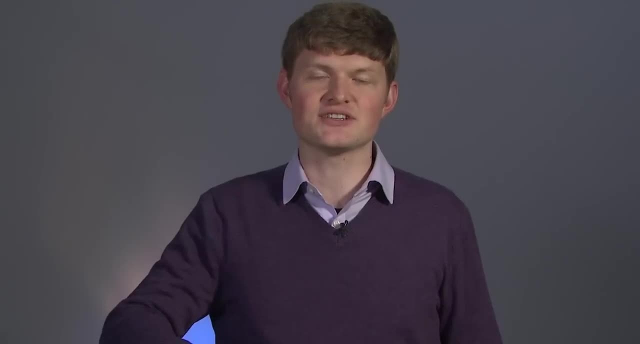 about the probabilities you encounter and consider how conditioning affects their interpretation. 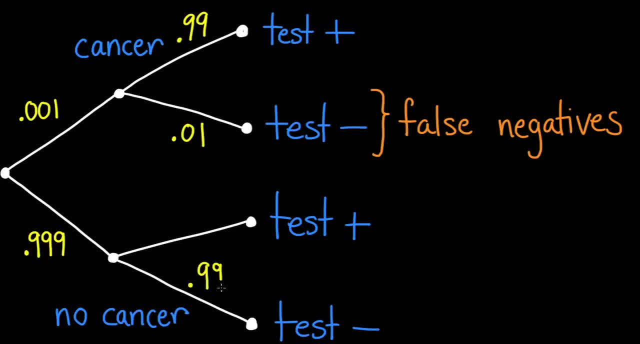 In the cancer-free population, 99% will test negative correctly, but 1% will test positive incorrectly. These incorrect results are called false negatives. These incorrect results are called false positives. Given that you test positive, our sample space is now restricted to only the population that tested positive. 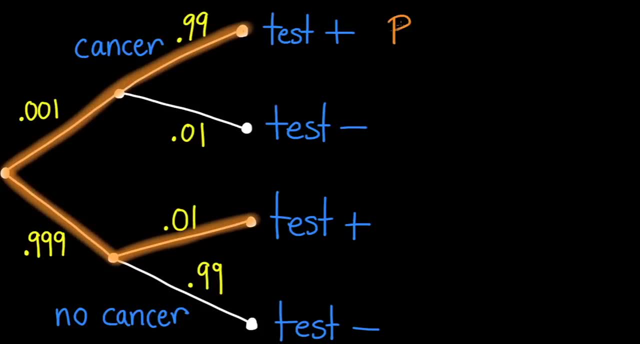 This is represented by these two paths. The top path shows the probability you have the cancer and test positive. The lower path shows the probability you don't have the cancer and still test positive. Now pause the video to determine the probability that you have the cancer. 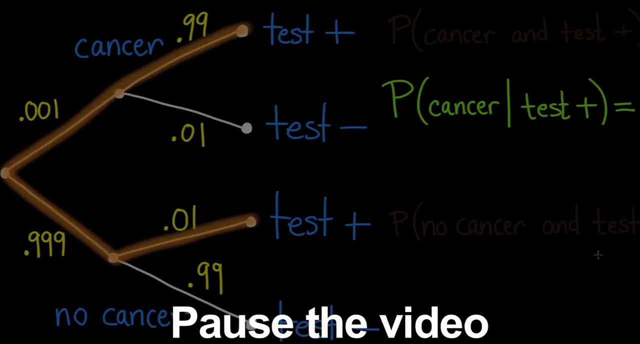 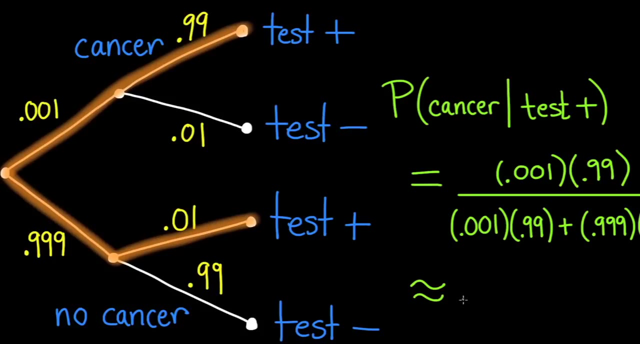 given that you test positive. The probability that you actually do have the cancer, given that you test positive, is given by the following expression, which works out to about .09, less than 10%. The error rate of the test is only 1%. 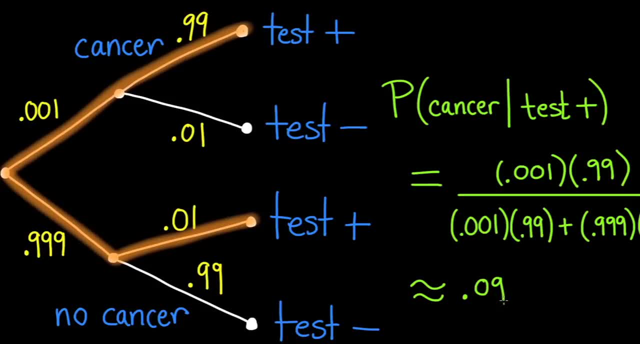 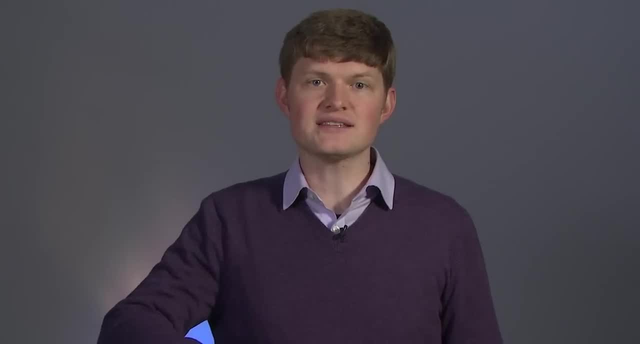 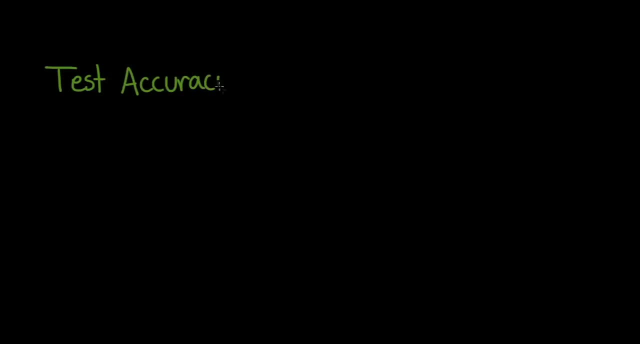 but the chance of a misdiagnosis is more than 90%. Chances are pretty good that you do not actually have the cancer, despite the rather accurate test. Why is this so? The accuracy of the test actually reflects the conditional probability that one tests positive. 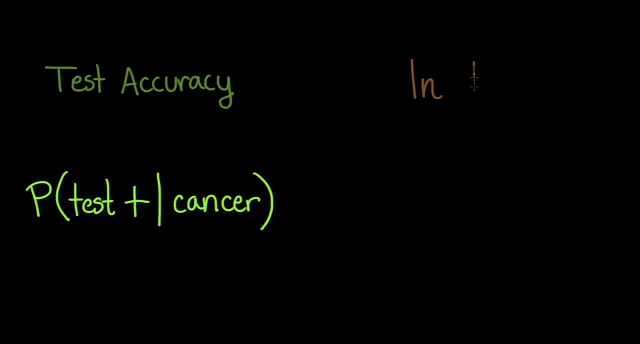 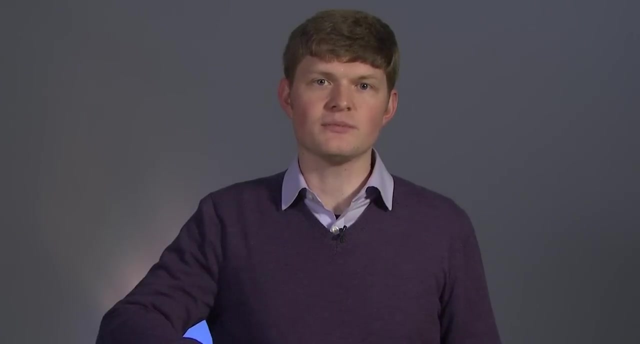 given that one has cancer. But in practice, what you want to know is the conditional probability that you have cancer, given that you test positive. These probabilities are not the same Whenever we take medical tests or perform experiments. it is important to understand. 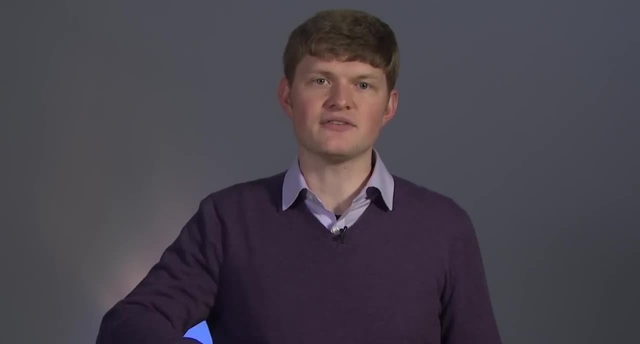 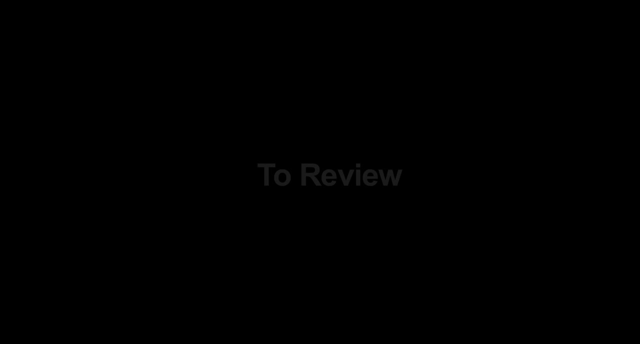 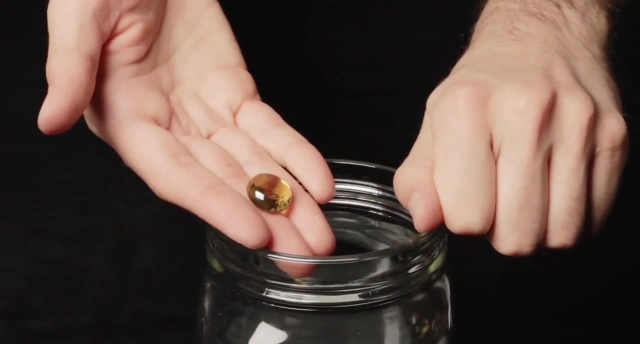 what events our results are conditioned on and how that might affect the accuracy of our conclusions. In this video, you've seen that conditional probability must be used to understand and predict the outcomes of many events. You've also learned to evaluate and manage conditional probabilities. 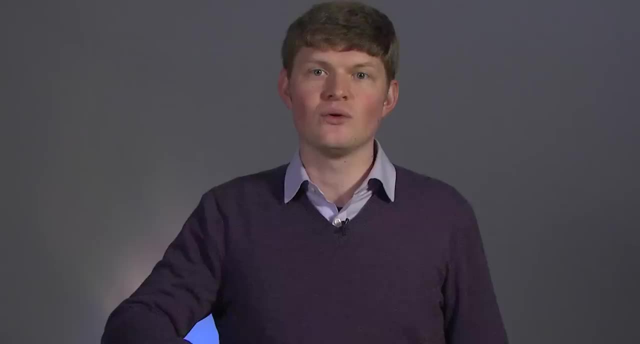 using tables and trees. We hope that you will now think more carefully about the probabilities you encounter and consider how conditioning affects their interpretation.